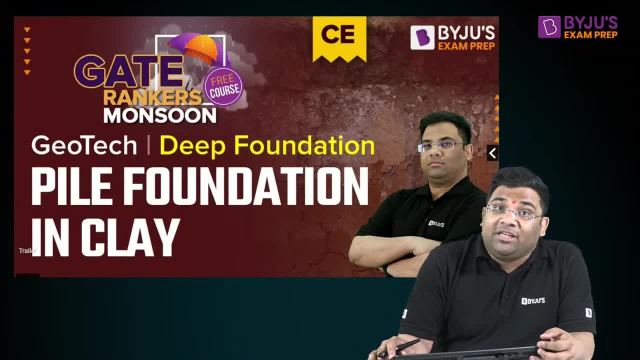 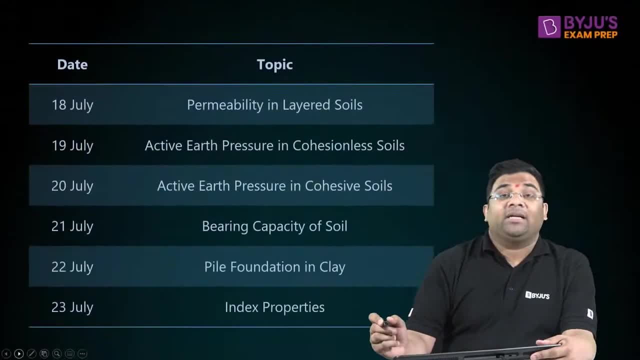 So today's topic is your pile foundation in clay. Okay, Pile foundation in clay. and let us go to the list of topics which we are covering in this particular video. Okay, So in this week- on Monday we started, we completed permeability in layered soil, Then we studied active earth pressure in cohesionless and cohesive soil. Yesterday we studied the topic bearing capacity of soil. That was for shallow foundation and in deep foundation we will see what Your pile foundation in clay. 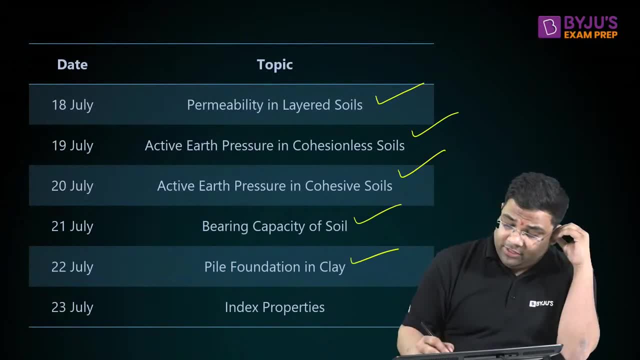 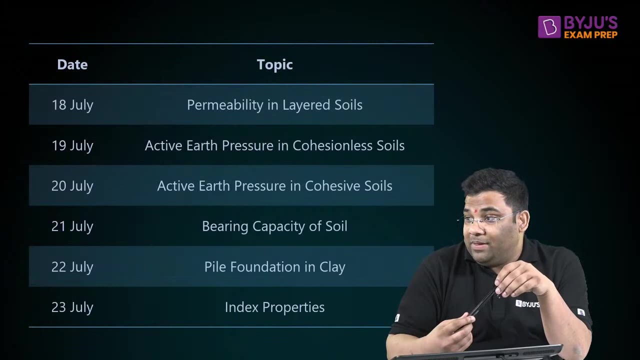 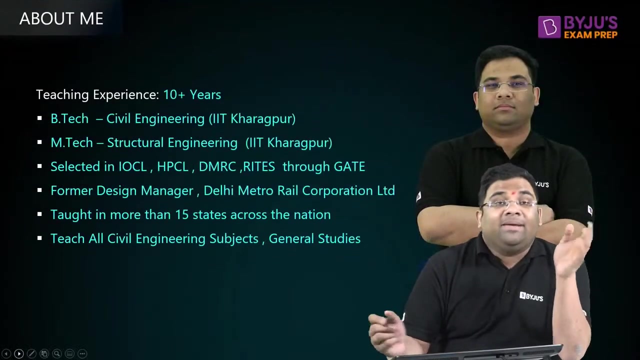 And tomorrow, that is, on Saturday, we will be studying what Your index properties. Okay, So let us start the lecture, but before that, let us welcome our friends. So welcome Karthikeya, Amit Kumar, Mukul, Juhi Rasmita Vivek and Saurabh Singh. Okay, So warm welcome to all the participants. Okay, And welcome to all the people or students who are seeing this lecture recorded also. So a short introduction about myself. My name is Satyajit Sahu. I have done my BTech and MTech from IIT Kharagpur. 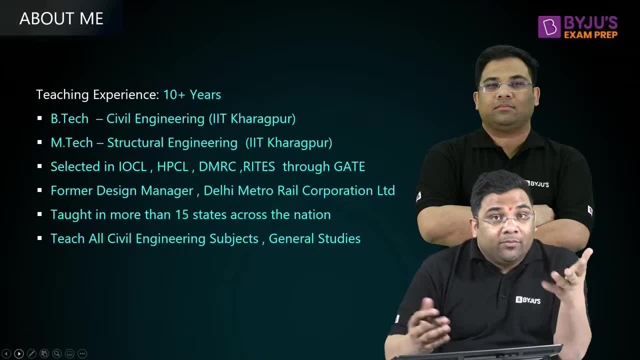 I have been selected into many PSUs through GATE and I have taught in more than 15 states and have a rich experience in GATE and ESE domain in the last 10 years, Okay, And I teach all the civil engineering subjects and I also teach what General studies for your ESE. So that is great. So let us start today's lecture, Okay, Without any further delay. My health is little down, Okay, So I will be taking little hot water in between, So please don't mind. 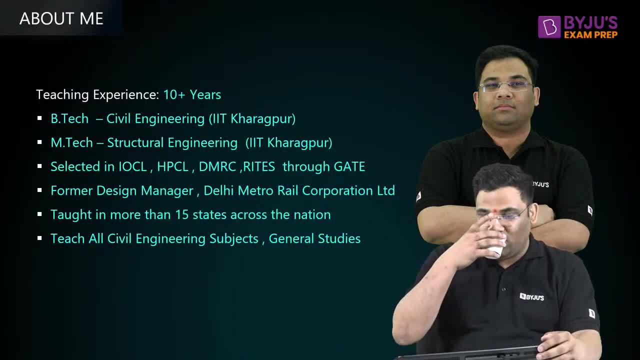 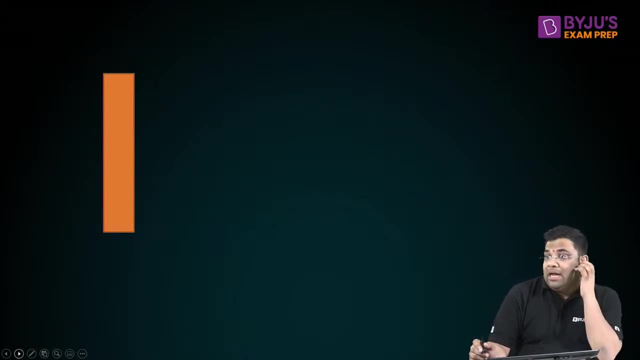 Okay, So we will have some water and then we will start the class. Okay, Thank you very much for this. Okay, So let us start the class. So this is a pile and pile is what Pile is a deep foundation. Pile is what Pile is a deep foundation. Now, yesterday we studied shallow foundation and how we define a deep foundation. 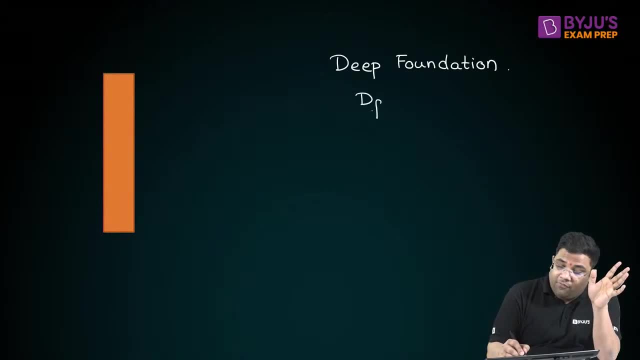 A deep foundation is a foundation where the depth of the pile or footing, I can say in this case, is more than the width or size of that particular foundation. You can see that this is the width of this particular pile, Right, And here. suppose this is the top of the pile and suppose this is at the ground level. Suppose this is at the ground level and this is the length of the pile. This is what 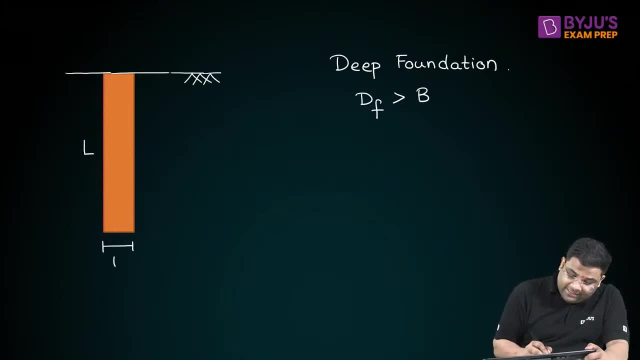 This is the length of the pile. So I can say that I can say that here the length of the pile is actually equal to the depth of the footing Right And you can see the depth is quite large compared to what The width. So here I can say it is a deep foundation. So the pile foundation is a type of what Is a type of deep foundation, Deep foundation. Now, what we are going to study in this pile foundation: 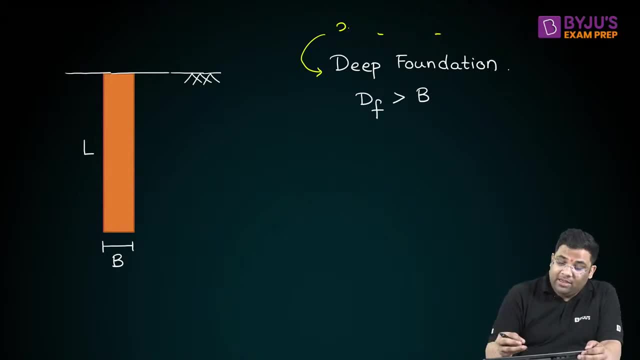 Okay. So piles are normally given when we have less bearing capacity for your shallow foundation. Normally we provide it for clay. Okay. So we are going to study today what Piles in clay. Piles in clay, Okay. Now you see, this is a single pile in clay. I can say: this is a single pile in clay, Okay. Now what we are asked in the examination is what? 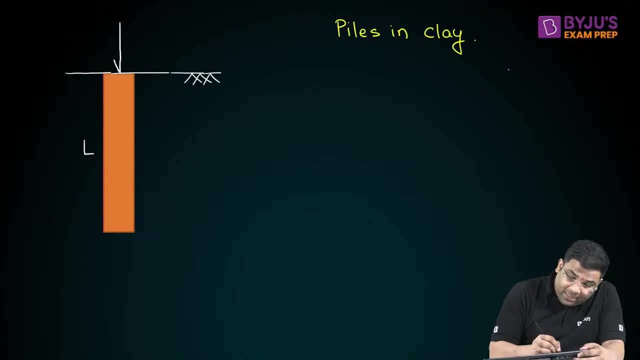 In the examination we are asked to find out the ultimate load carrying capacity of this pile foundation, Ultimate load carrying capacity of this pile foundation, or I can say single pile in this case. So what is your QU? Your QU is the ultimate load capacity of the pile, or I can say ultimate load which the pile can take. So ultimate load, I can say. 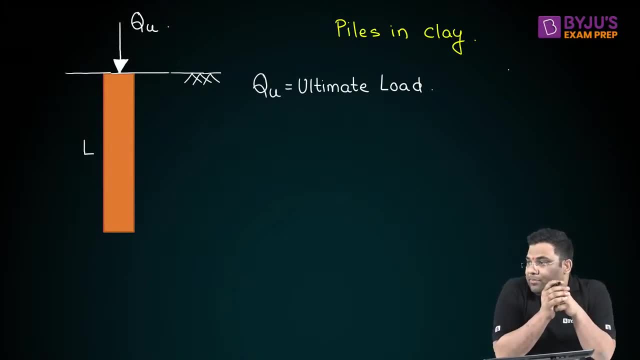 can say in short, I can say: what Ultimate load. Welcome Saurabhsri, Vijit and Aptap. Okay, So ultimate load. Now, this particular load will be registered by two things. So I can say: two resistive forces. One resistive force will develop at the base. Yes, One resistance. 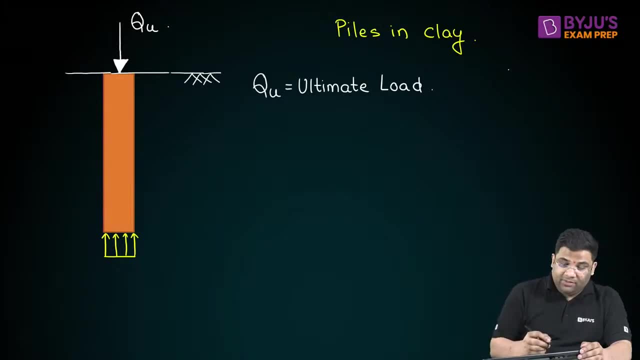 will be coming from the base. Another resistance will be coming along the faces, or I can say side of this particular pile. So two type of resistance this particular load QU will face. So two resistance, Okay, Two resistance, One at the base, Other one is along the surface. 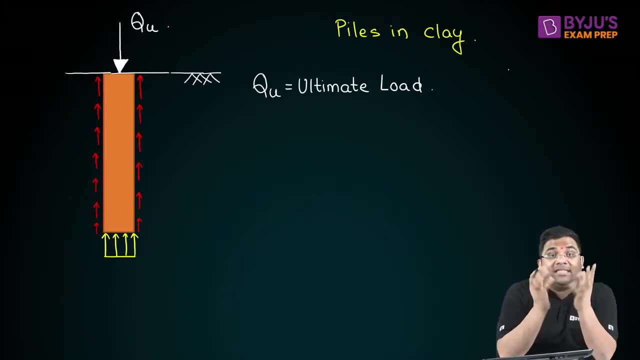 Another one is along the surface, or I can say, faces Right Now. this is the base. This is the base I can say. Therefore, I will call this as end bearing resistance. I will call this as what End bearing resistance. It is known as what End. 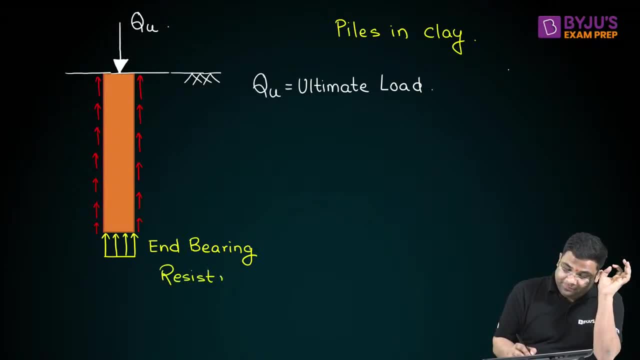 bearing resistance. Okay, And the one coming in the side. I will call that as what? Your frictional resistance. I will call that as what? Frictional resistance. So this ultimate load. So you will have two types of resistance. One is the end bearing resistance, The other 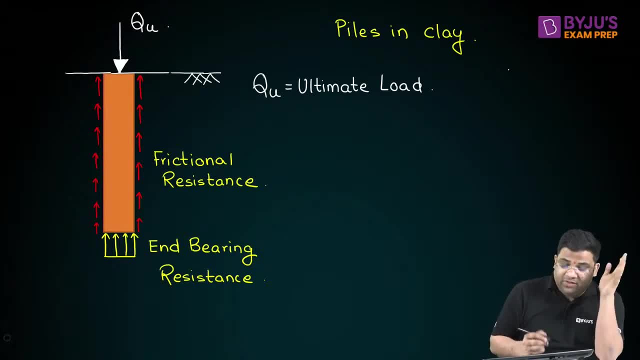 one is frictional resistance. Okay, Now, this frictional resistance can be also told as: what Screen frictional resistance? Because it is coming along the skin or surface. I can say, Right Screen frictional resistance. This I will give a name QF- F for friction. 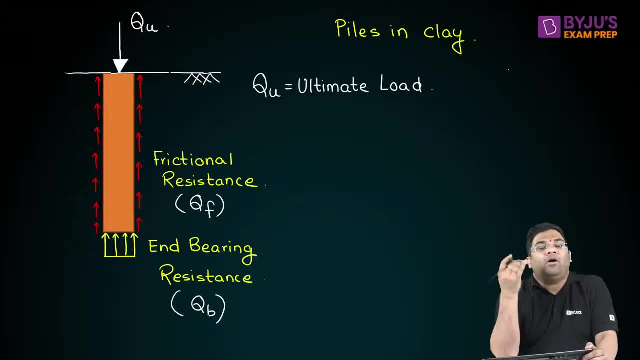 and this I will give the name QB, B for your bearing resistance. So now you can see, And this will be the load, So this will be a load- You will see that this ultimate load will be balanced by this Frictional resistance and 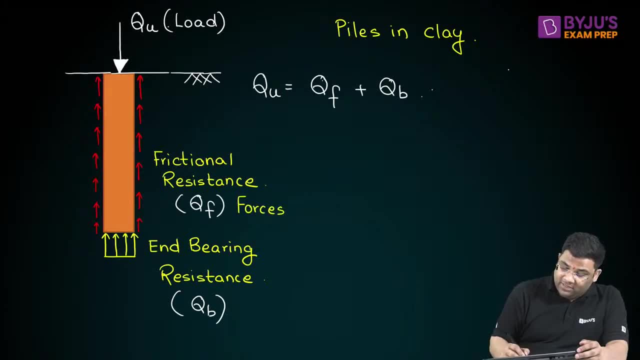 your end bearing resistance. Welcome that. So Frictional resistance and end bearing resistance. Now see this: Q is actually a load. It is a load. So I can say your QF and QB also will. They are forces. They are what They are forces. So if I am taking them as force, I am taking them as force. What is force? Force is simply the stress into your area, right? 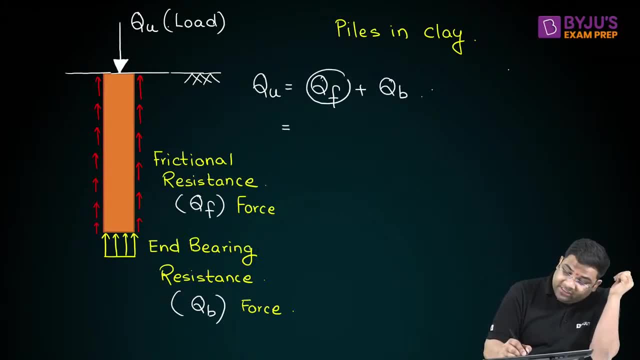 So here I can write down this as the frictional resistance force, as the frictional resistance stress into area under friction- Yes, Plus the end bearing stress into what Area of base Load is. what Load is your stress into area? I just use that Right. 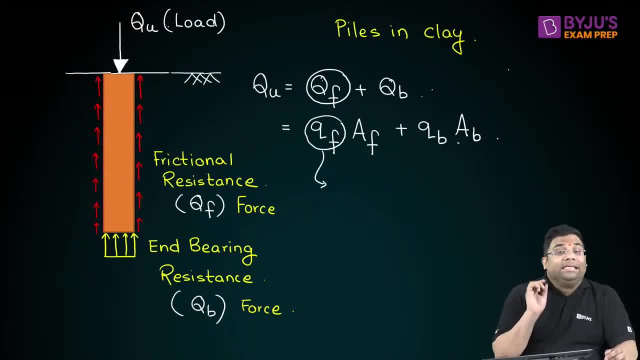 So this is known as what? This is what, This is your frictional stress. I can say, This is what The frictional stress Right, And this I can say is: end bearing stress. It is what? End bearing stress. Okay, End bearing stress. 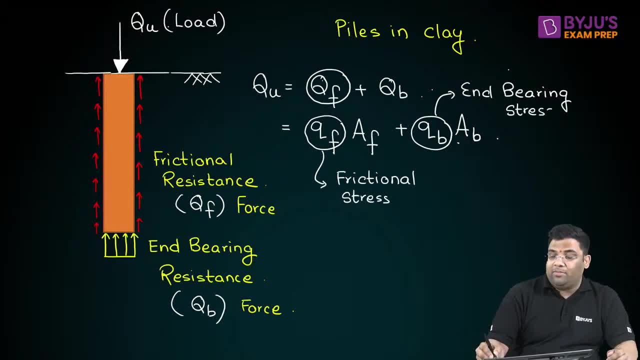 We will come to that. We will come to that. Okay, In some time we will come to that. The end bearing stress and the frictional stress. But what about these areas, These frictional areas and the basic? Try to understand. Suppose this is a pile. This is not a pile. Just imagine this is a pile. You can say: this is what This, I can say, is the frictional area. Right, 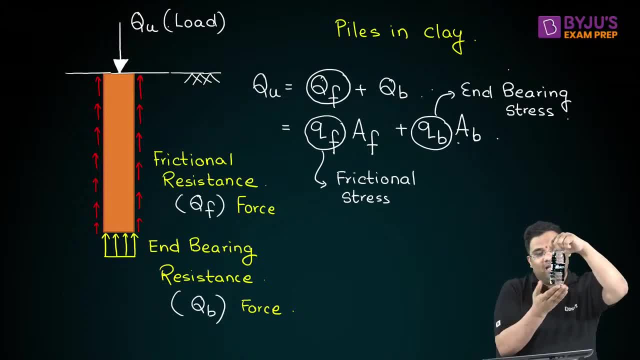 Suppose a cylindrical thing, This is a frictional area, Whereas this is what. This is the base area. It is very common sense. Right, It is the base area and this is the frictional area. And I can say: ultimate load is applied like this. Right, It is, the ultimate load is applied like this. 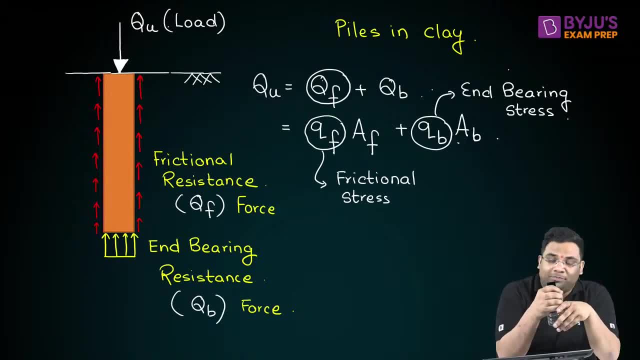 And I can say: ultimate load is applied like this. Right, It is very common sense, Right It is the ultimate load is applied like this. So this is the QU, This is the frictional resistance and this is what This is, the bearing resistance, or end bearing stress, I can say Okay. 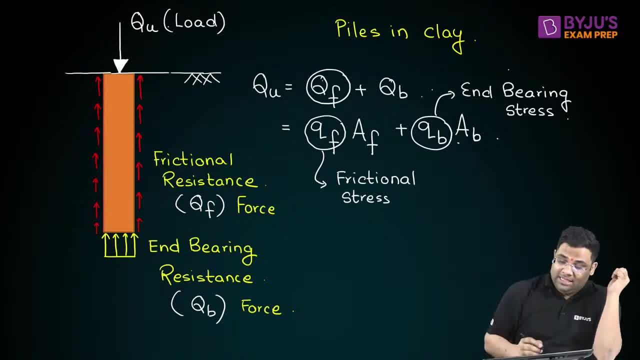 So we will come to the stress values later on. You see this frictional area, This frictional area, I can say the surface area, Right? Yes, This is frictional area, I can say surface area. And this bearing area, It is the base area, Right? 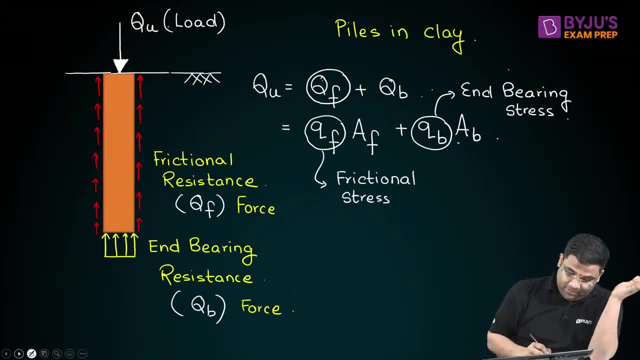 Now this surface area or frictional area and the base area will depend on the shape of pile. We will depend on the shape of pile or cross sectional shape of pile. So we adopt normally to cross sectional steps. Okay, The normally adopt to cross sectional steps. 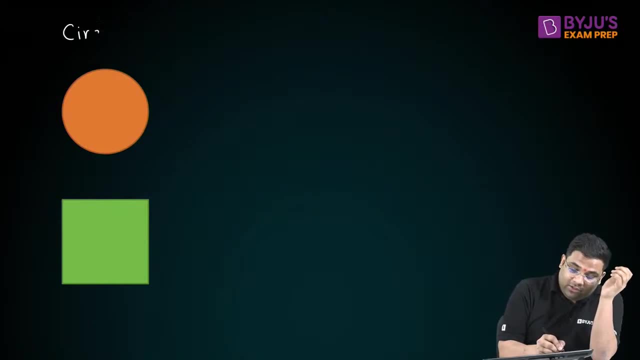 The first one is what we adopt- a circular cross section- or we adopt what? A square one, a circular one or a square one. So no need to remember the formula. If you know the basic things of geometry, you know. I told that your frictional area is nothing but the surface. 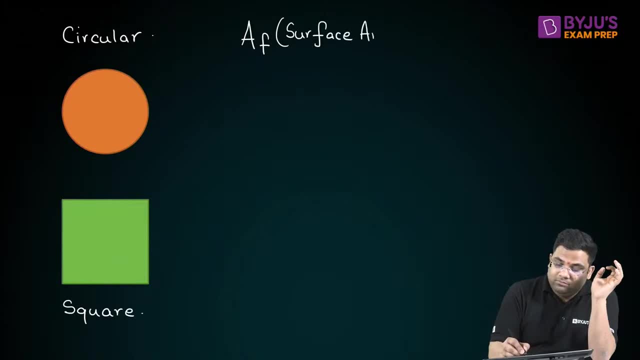 area. right? Yes, this is the surface area. I write down in the bottom surface area: It is the surface area And AB is your base area. So tell me, you only will tell me. I will not tell. you will tell that if this is the diameter of the circular cross section, 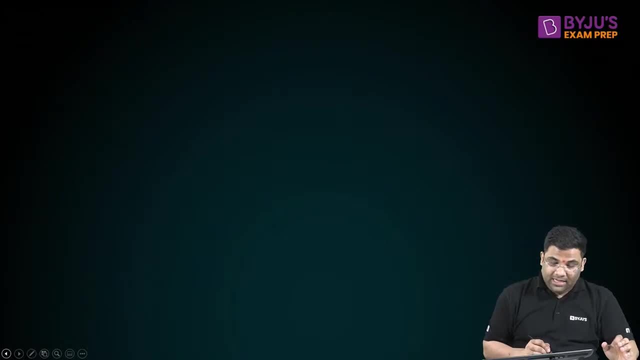 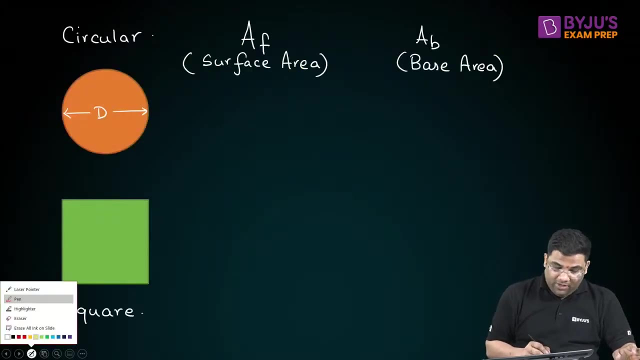 and L is the length of the pile and L is the length of the pile, like this, then, can you tell me, can you tell me what will be the surface area? What will be the surface area? You see, this is circular cross section, right, This is. 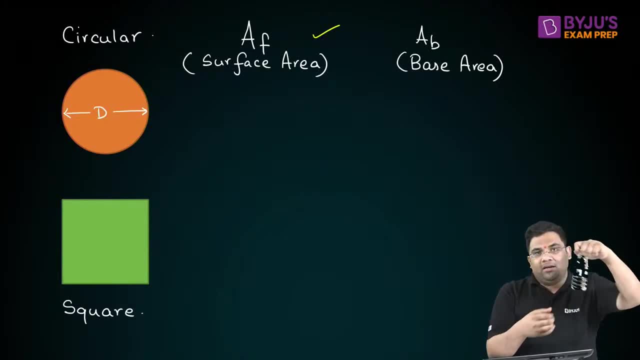 circular cross section. What will be the surface area? Can anybody tell? If the diameter is D, what will be the surface area? Please mention. Till that time I will have some hot water. Very good, very good, very good. Others also write down in the comment section what will. 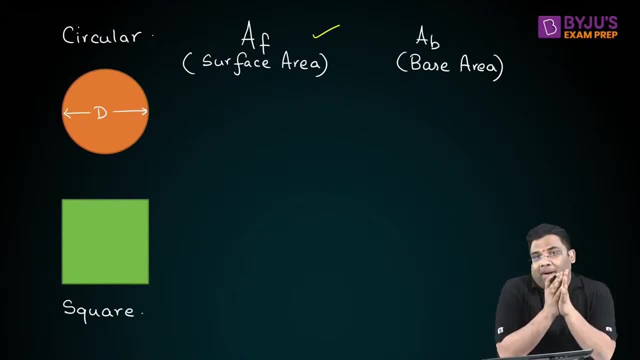 be the surface area Of this circular pile. Surface area of the circular pile. See, need not remember the equation, You can just use your common sense. Others also write pi D, L. Very good, Surface area will be pi D into L. This pi D is the perimeter right. This pi D is the perimeter. 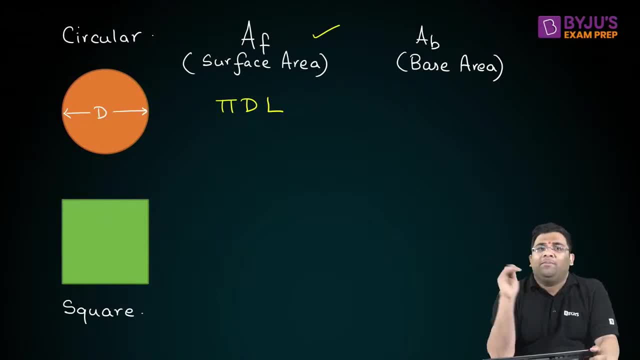 and then length. That gives me the surface area. What will be the base area? Write down the base area. You will write down everything. I will just, you know, guide you. So this: Tell me what will be the base area for your circular cross section, For your circular. 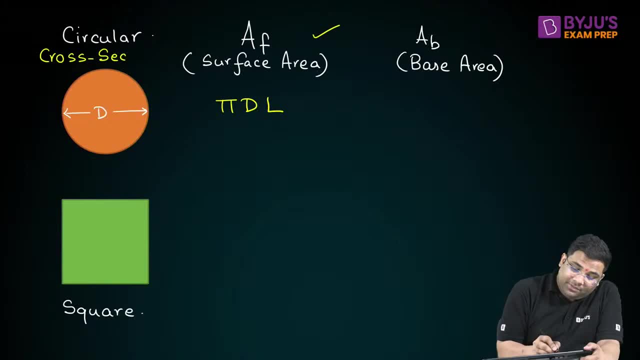 cross section. what will be your base area For circular cross section? what will be your base area? Yes, pi D squared by L. Yes, Pi D Round by 4, pi D square by 4.. So you see, it is very simple. Base area: pi D square by 4,. 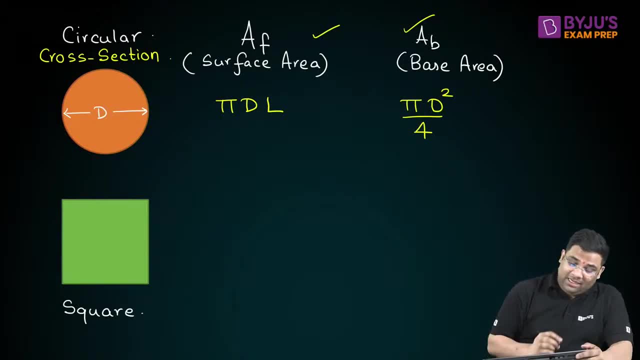 surface area: pi D into L right Now. similarly, if the square has a side length of B. similarly, if the square has a side length of B, then tell me what will be the surface area, what will be the base area. Please tell me what will be the surface area, what will be the. 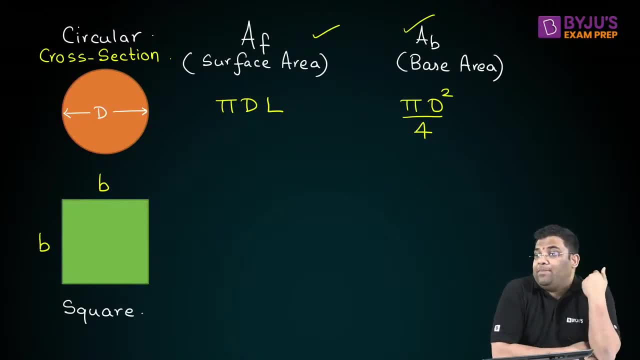 base area for square In one go. you tell me the base area and the surface area for the square. okay, For the square base area and surface area, Please write in the comment section. You might be thinking sir is teaching so simple things because in the examination 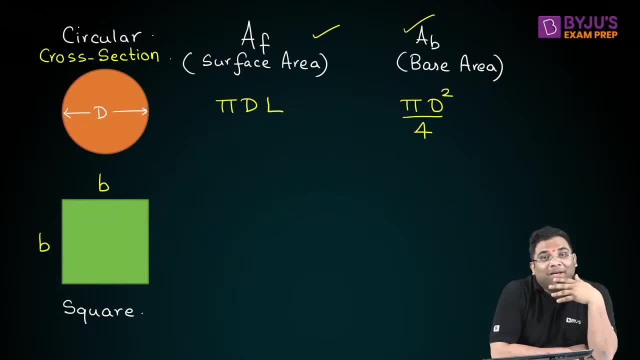 they ask you simple things. only We just do not know that things are simple. What is the surface area and what is the base area for a square pile? Yes, Gorang is writing 4B square, 4B square. It will be 4B into L right, 4B into L, Okay. 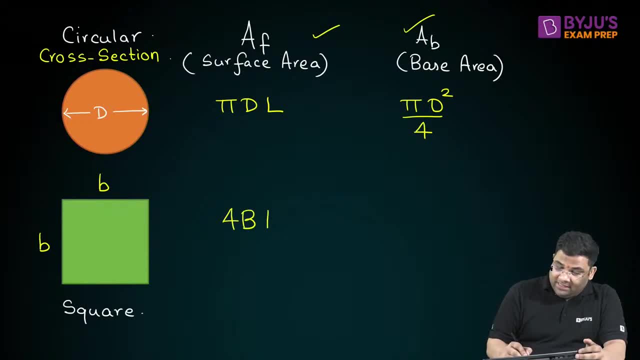 very good. 4B into L, the perimeter into length, the surface area and base area will be simply B square. So if they give the cross section, okay, if they give the cross section, we can easily find out what. 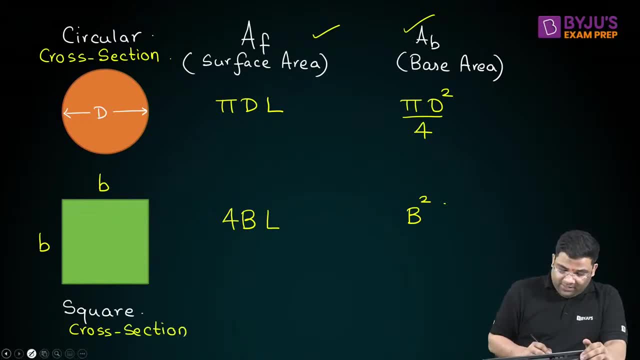 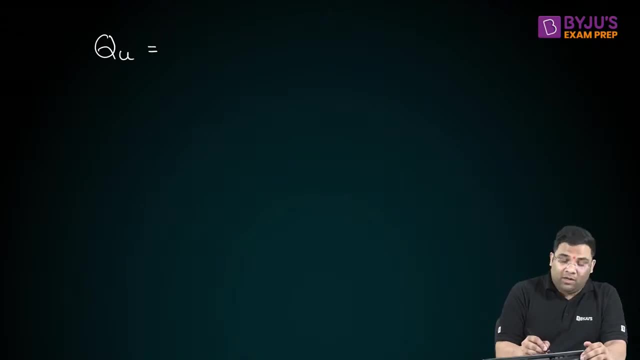 This base area and the surface area, Then what is remaining? What is remaining is the stresses. So we saw the ultimate load is equal to the frictional resistance plus the end bearing resistance. Now the frictional resistance is the load. It will be the frictional. 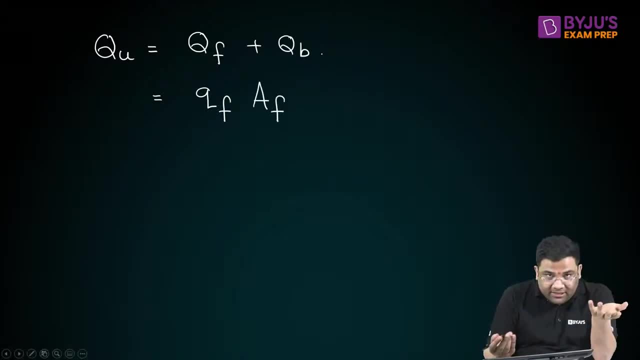 stress into the area under friction Area. under friction is the surface area that we saw, plus your end bearing resistance into area. So what is remaining? What is remaining is this: yes, What is remaining is this and this. So, how to find out these two things, I will tell you, do not worry, You see this. 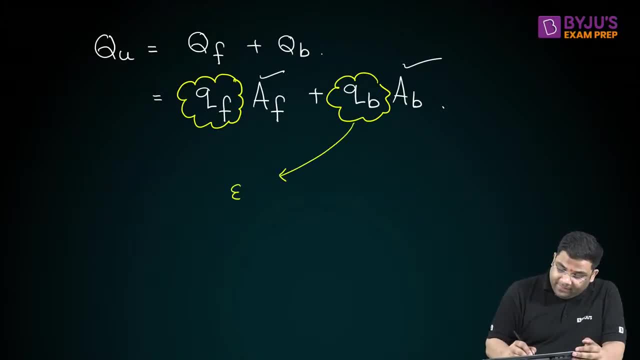 is your end bearing, This is what This is your end bearing, End bearing stress. I can say, I can say this end bearing stress is nothing but the frictional resistance. This is the frictional resistance, This is the frictional resistance, This is the frictional resistance. 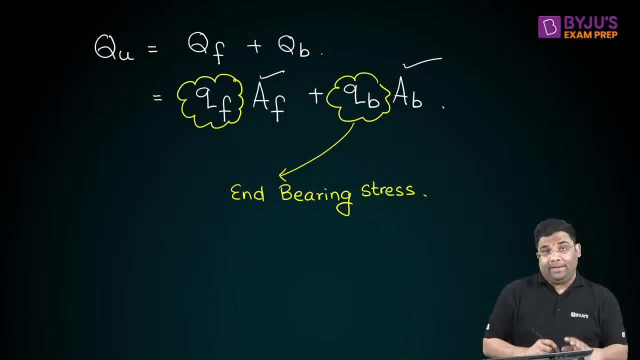 Now, this is nothing but the bearing capacity, nothing but the bearing capacity. Now, bearing capacity is what C and C plus Q and Q plus 0.5B gamma and gamma Right, 0.5B gamma and 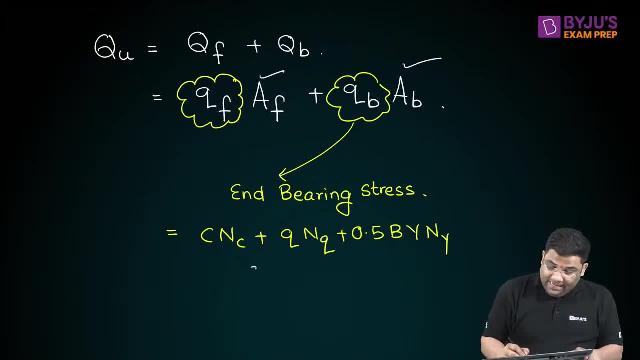 gamma. Now, since it is a clay, the n gamma becomes 0.. Clay means n gamma becomes 0, ok, And this particular NC will become 9.. Now, yesterday we learnt that NC is equal to 5.7.. 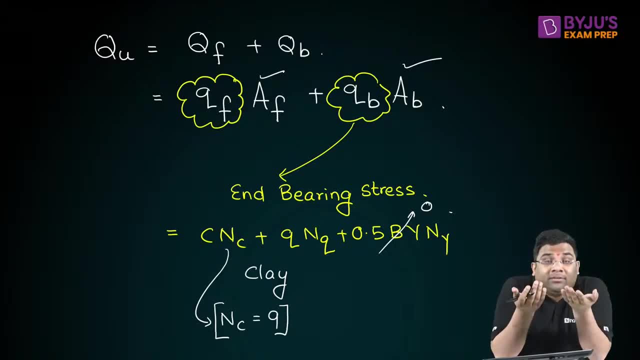 That will be applicable for shallow foundation. You see, deep foundation. this particular pile is a deep foundation And that case NC will be 9.. So NC is 9 and this term is less. I can ignore this and make it 0.. 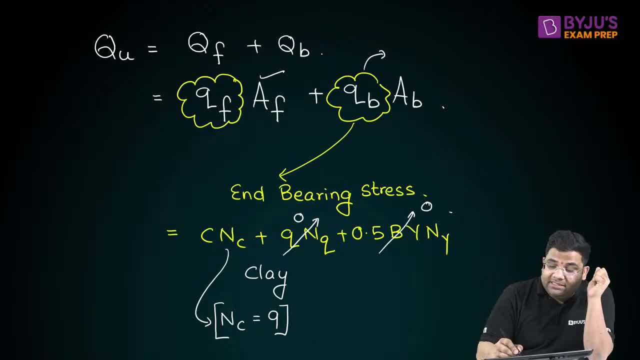 So, simply, your end bearing resistance comes, what With 9 into C, 9 into C. Now your frictional resistance depends on cohesion. It depends on the cohesion. You see, this particular pile. suppose This pile will be embedded inside what? 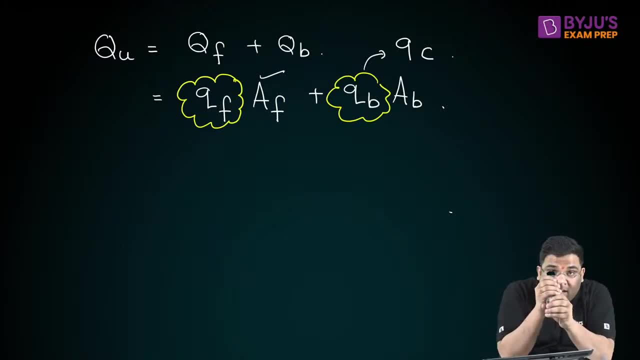 It will be embedded inside clay, So the surface of the pile, the clay will be attached. right It is embedded inside clay, So clay will be attached. So tell me, between the clay and the pile there will be adhesion or cohesion? 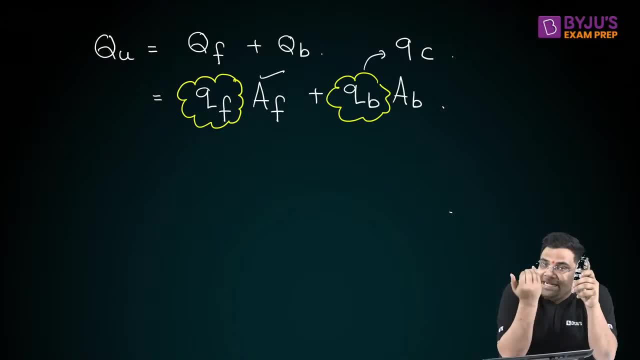 Between the pile surface and the clay there will be adhesion or cohesion. Please mention in the comment section. But between the pile surface and the clay there will be adhesion or there will be cohesion. There will be adhesion And that adhesion will depend on what. 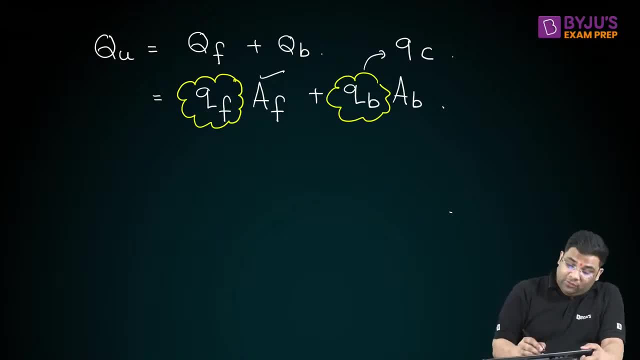 That adhesion will depend on the cohesion value. So I will write this as alpha into C, where C is your cohesion, Where C is your cohesion and alpha is your adhesion factor, Alpha is your adhesion factor. So now I can say the ultimate load is equal to alpha into C, into the frictional area or I can say surface area. 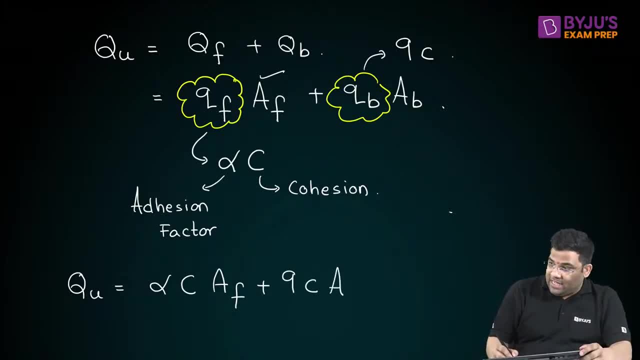 Plus nine into C, into area of piece curse. Very simple formula. Again, remember this formula by the explanation which I gave you. Very simple, Okay, Thank you. So now next thing is: what Next thing is? we will solve a question. 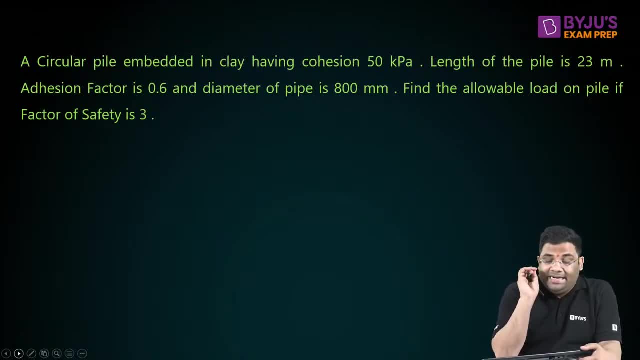 We solve a question. Okay, So a circular pile embedded in clay having cohesion value 50 kilopascal, So cohesion is 50 kilo Pascal, So cohesion value: 50 kilo Pascal, So cohesion value: 50 kilo Pascal. 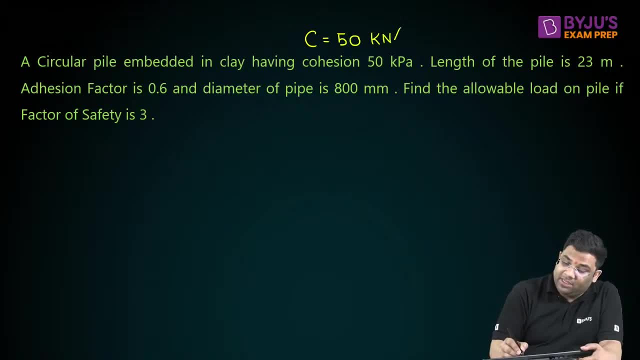 is given to us 50 kilo. Pascal means 50 kilo Newton per meter square. Length of the pile is 23 meter. Length of the pile is 23 meter. Alpha is given to us as 0.6.. Alpha is given. 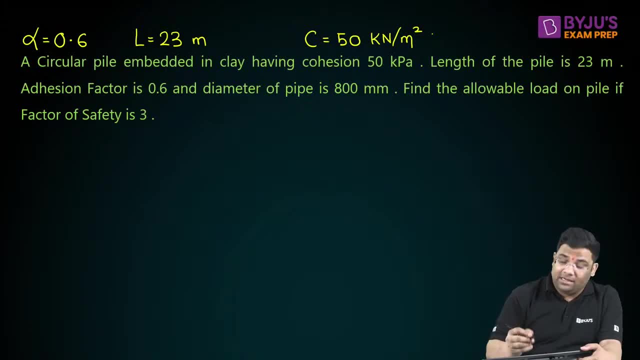 to us as 0.6.. Diameter of pipe is 800 mm, So diameter is 800 mm. Find the allowable load on the pile if factor of safety is 3.. Now see, it is very easy. See first of all, allowable load. will be what Allowable load? How to find out allowable load? Take the ultimate. 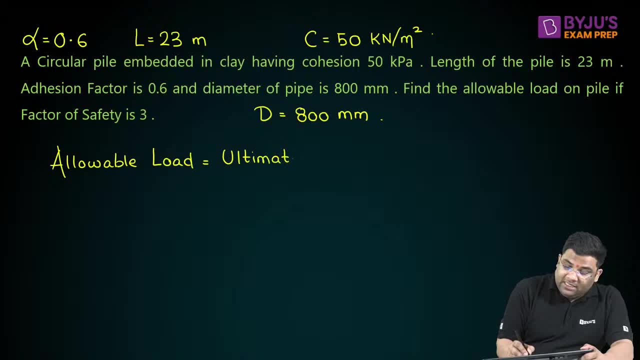 load and divide it by factor of safety. See ultimate load is what? How much maximum it can take? But you will not allow that much Now. you will allow less than that right. So divide by the factor of safety And factor of safety is given as 3.. So now this is equal. 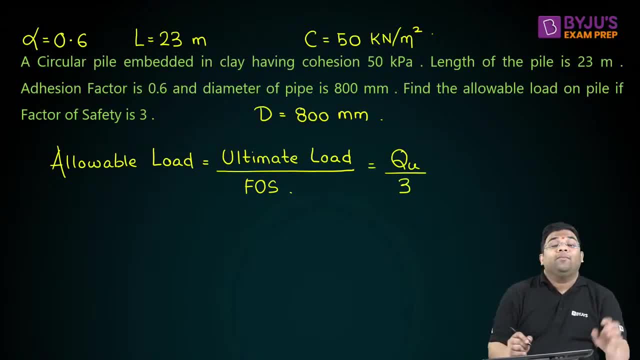 to the ultimate load Length of the pile divided by 3.. But for this to find out allowable load, I need to find out what The ultimate load, Your ultimate load, is, what That is equal to the frictional load resistance plus what The end bearing resistance. Now this is equal to the frictional 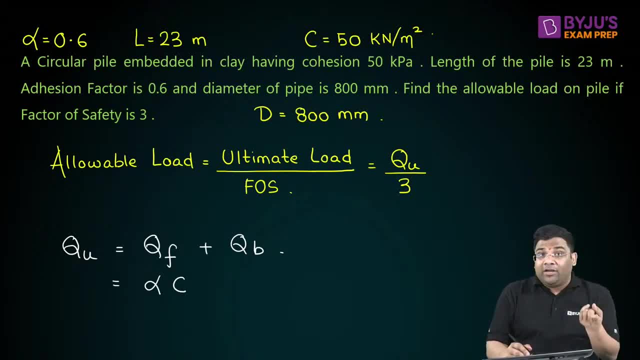 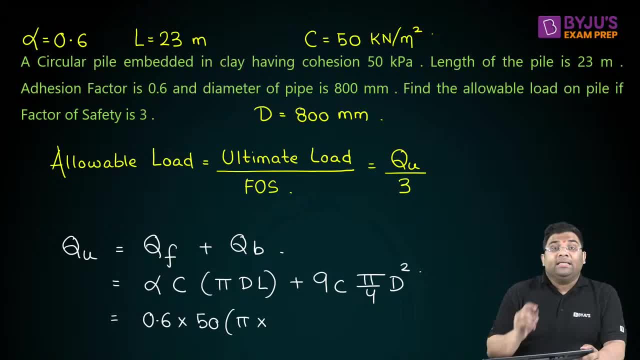 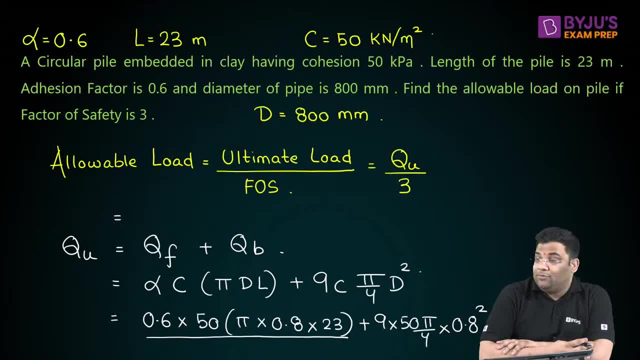 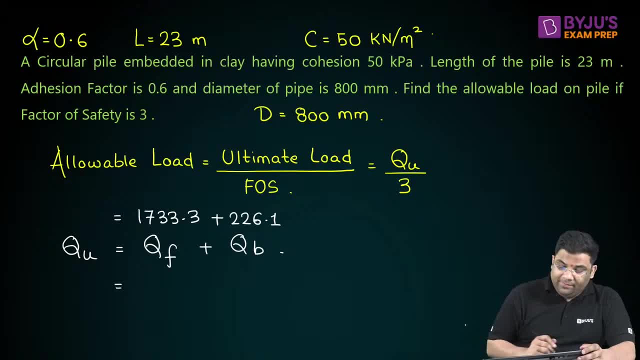 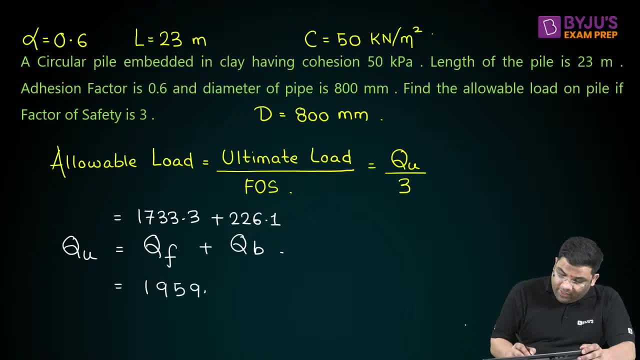 Will be 1959.4 kN. right Will be 1959.4 kN approximately. We have done some approximations and that is perfectly fine. Now your allowable load will be 1959.4 divided by 3.. 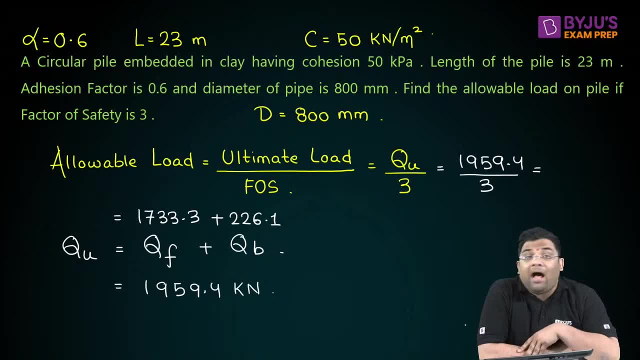 Giving me how much? As our very dear Apta found out, It is your 653.12. you are getting. Getting how much 653.12,? I can say 1,, 3, almost. I am getting Understood this question. 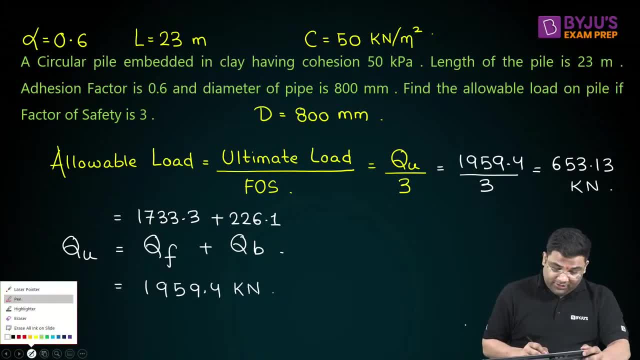 It is a very straightforward question, but they can ask you such questions. Okay, Now in the examination, be little careful. What care you have to see Sometimes they will not ask you to find out the ultimate load, They will just ask you what. 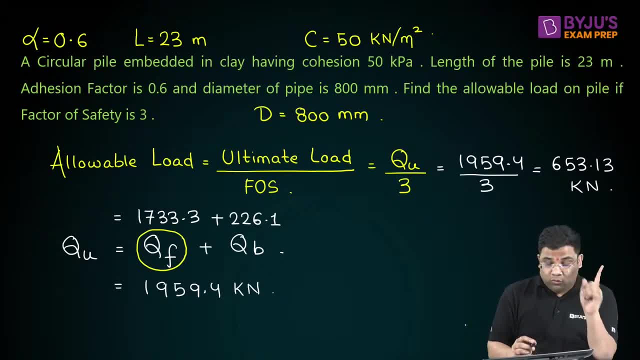 Find out, Find out the screen frictional resistance. If they ask you only find out the screen frictional resistance, This is the first type of question they can ask. So just mention, and this is the answer, The first type of question they will ask. 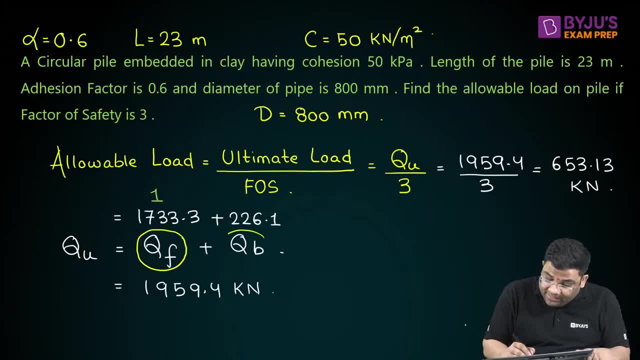 Find out the screen frictional resistance. Or they will ask you the end bearing resistance Right, Or they will ask you the end bearing resistance- Second type of question they will ask. So in the examination, be little attentive that they are asking you screen friction or end bearing or the ultimate one. 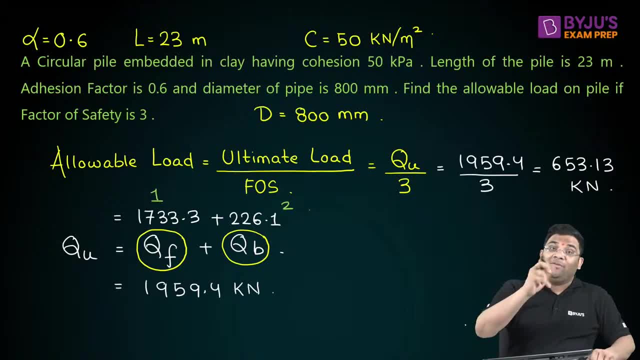 Okay, You have to see, Sometimes they ask you individually also: Okay So, and sometimes they will ask you directly the ultimate one. So ultimate one is this, And sometimes they will ask you the allowable one. So you have to be very careful what they are asking you in the examination. 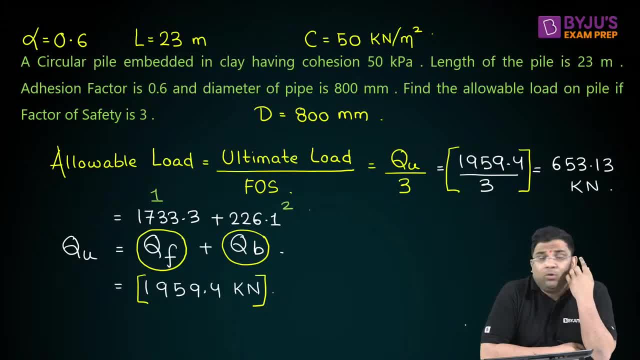 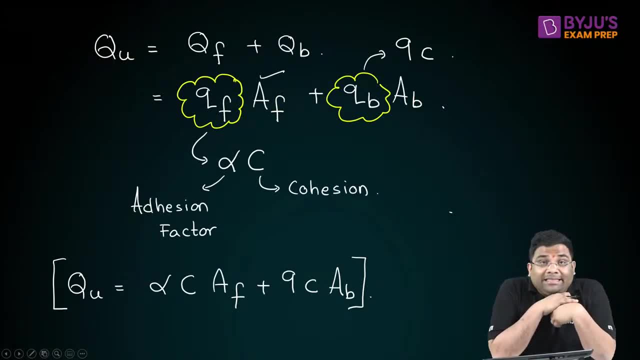 Easy. It is a very straightforward, simple question. Now, if you see this equation, there are so many things Right. You see, there is cohesion, There is alpha, There is what in this area? There is what diameter length, side length. 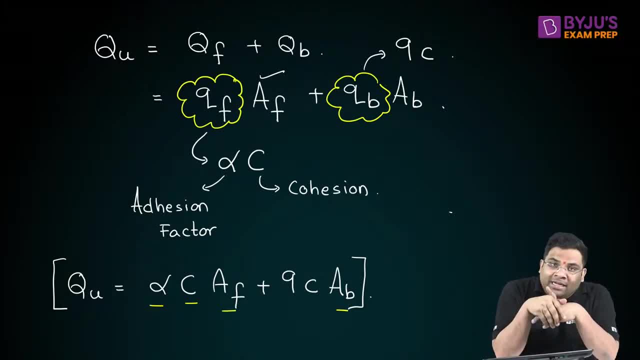 Right. So what they might do, They might give the ultimate load, Right. They might give the ultimate load And then ask you to find out any one other parameter, Like, suppose, alpha, they will ask you, Or cohesion, they will ask you. 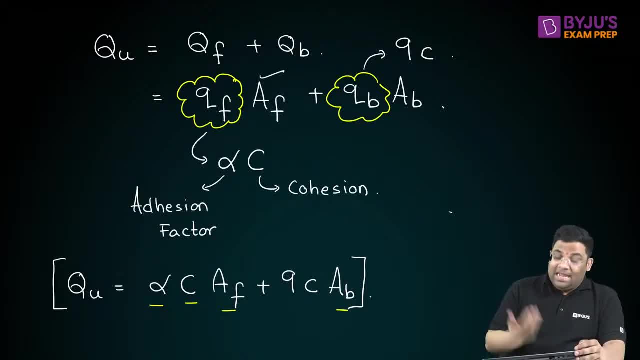 Or they will ask you what The length of the pile, Or they will ask you the diameter of the pile. Okay, So such questions also they will ask you. The equation remains same. The equation remains same, Just the unknown quantity will be different. 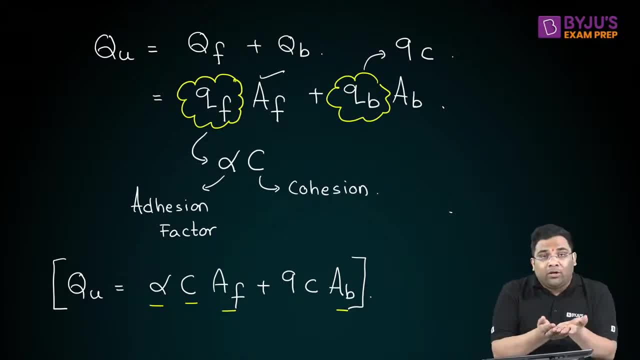 Equation same. In this particular question we found out the ultimate load, But in the examination they might ask you to find out ultimate load, Or they will give you the ultimate load And then ask you to find something else. Let us solve the question on this. 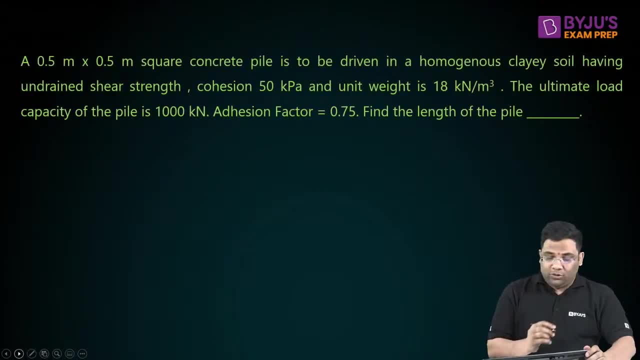 Okay, So this is the question, This you will solve. So this, Solve this. Okay, I will give you some time, So solve this. Okay, Let us see how many solve this question properly: 0.5 into 0.5 square concrete pile. 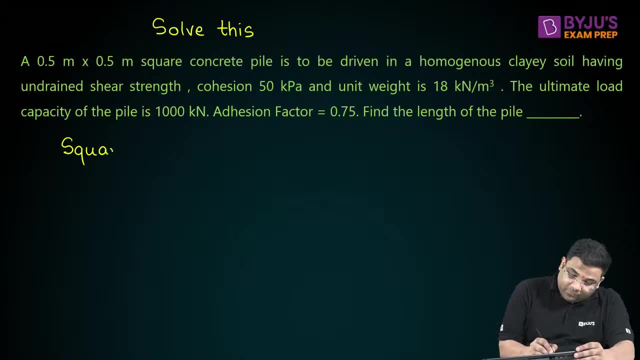 So it is a square pile. 0.5 into 0.5 means what This is, what This is. your side length Is to be driven into a homogenous clay soil having undrained shear strength, cohesion- how much? 50 kilo Pascal? 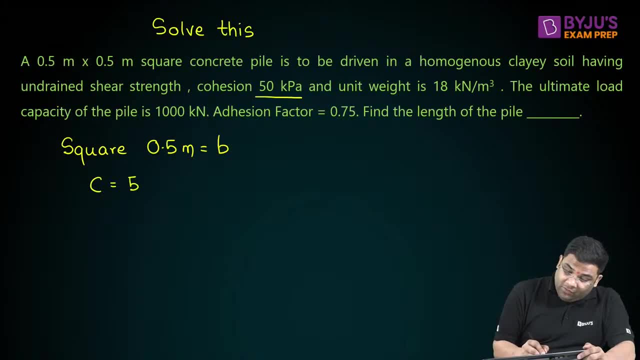 So the cohesion is given as 50 kilo Pascal. The unit weight is also given. Okay, The ultimate load capacity of the pile is 1000 kilo Newton. So Q is given. It is given how much 1000 kilo Pascal. 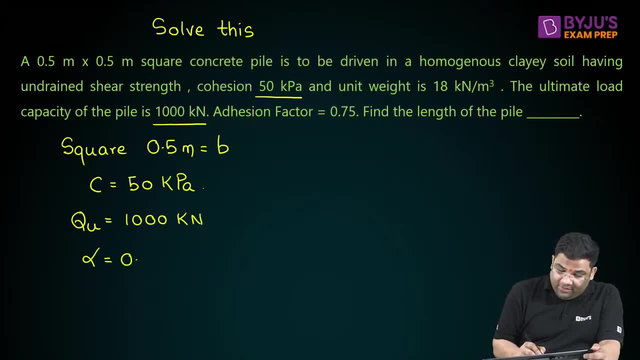 The addition factor is given as 0.75.. It is given how much: 0.75.. You have to find out the length of the pile, Okay, So please solve this question. I will give you some time. Please solve this question. 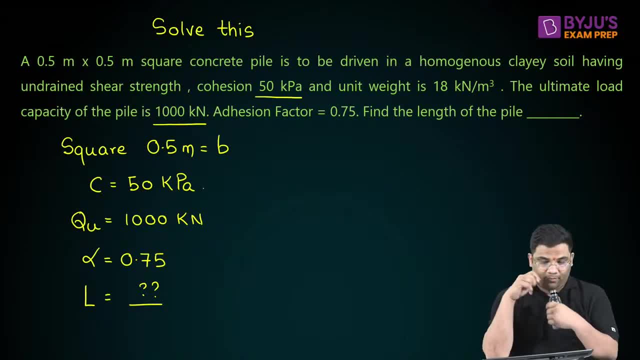 Let us see how many are able to solve. I will have some water. Thank you, Okay. Aptab found also Very good. Others, please find out. Some students are my old students, So they will be able to solve the question faster. 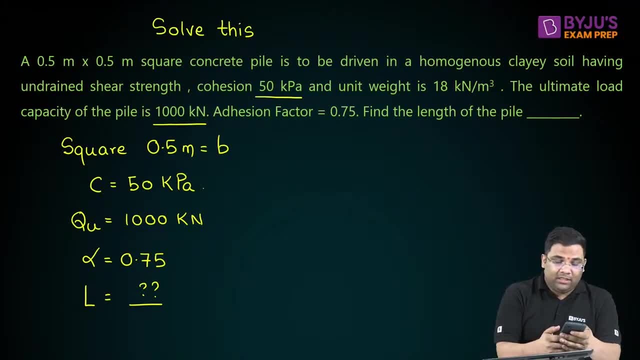 So I have the same question. Okay, So I will give you some time. Okay, they will be able to solve the question faster If you are taking time. no need to become disheartened If you are learning it for first time. 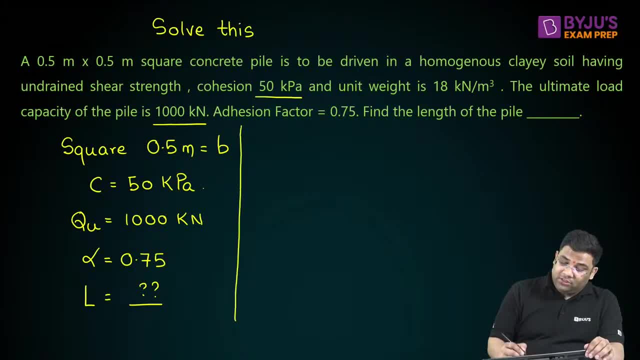 it's very obvious that you will be taking time to solve the questions, So don't get disheartened. Aim is to understand the concept and solve it fast. Aim is to understand the concept and solve it fast. If you are taking time for the first time, that is okay. 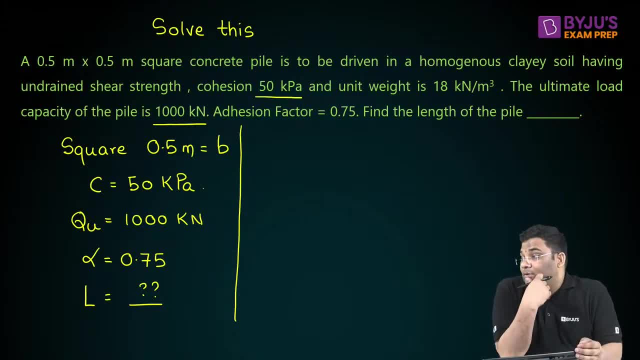 So no issues if you are studying it for the first time. So many students have answered the question. I will wait for others also to answer. I will wait for. Thank you, Bhaskar, So I will wait for other students to answer. 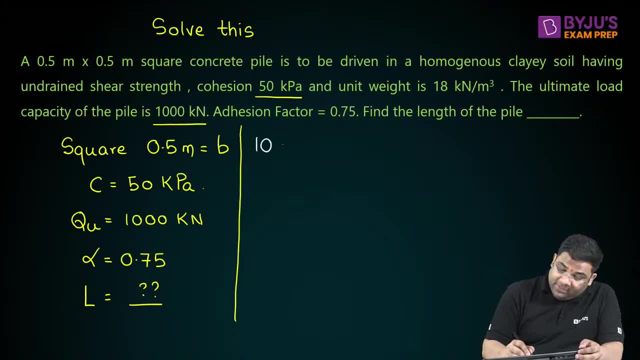 Okay, So let us solve this question. You see, the ultimate one is given 1000.. This 1000 will be equal to what The formula comes into picture Here. it is a square file, So friction will be alpha into C. 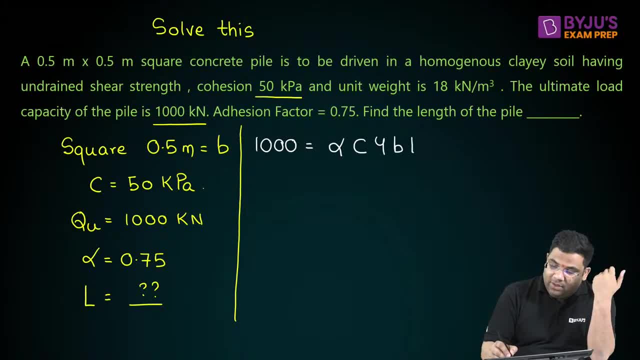 Then the surface area will be how much 4 times B into L, Plus what Your 9 into C, into what Area of base? Area of base will be B square here, Right? So from here I can say 1000 will be equal to alpha is 0.75.. 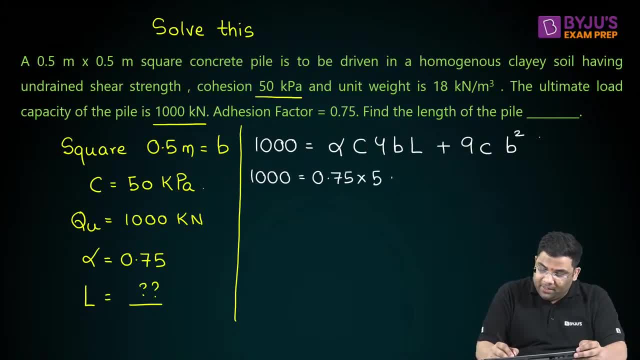 Cohesion is how much Cohesion is given as 54 into B. Now the side length is given 0.5 meter, So 0.5 into length, Plus 9 into 40. Or 50, sorry, 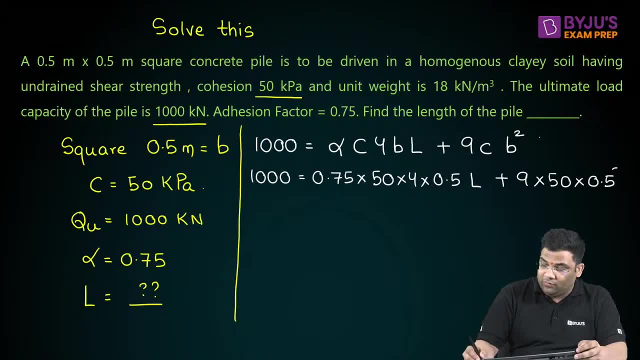 50 into B square means what 0.5 square. So this is 1000.. Solve it very systematically. This will be how much? 200 into 0.5.. 100.. This will be 75 L, I think. 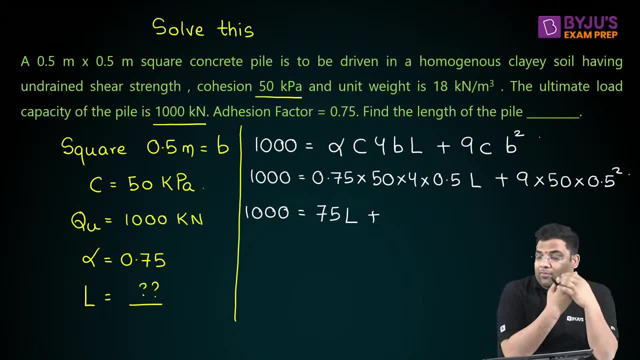 Right, It will be 75 L Plus 0.5 square will be 0.25.. 0.25 of 50 will be 12.5.. 12.5 into 9.. 12.5 into 9.. 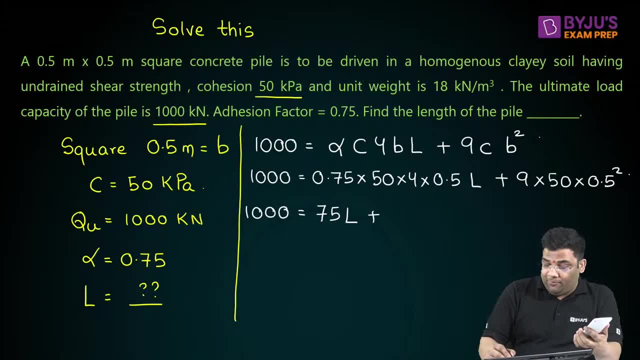 Will be 112.5.. Okay, So from here, L will be equal to 1000 minus 112.5 divided by 75.. Okay, Just some error. Okay, So we are getting 11.83.. So again, you see, it is a very straightforward question. 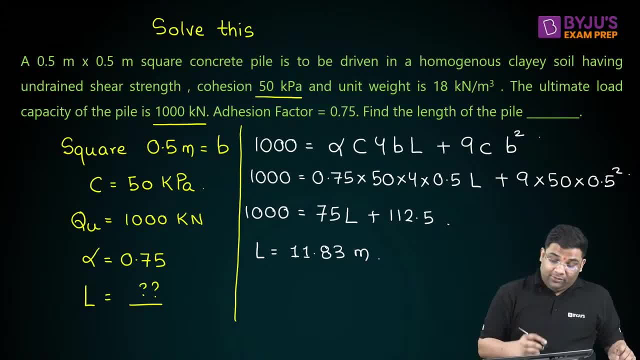 You just need To apply the formula properly. You see, here length was given. They could have asked cohesion, also right. Or they could have asked you find out the alpha by giving other values. Or they could have asked you find out what? 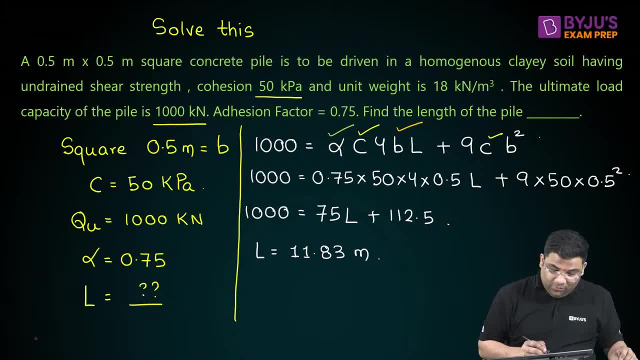 This width Right? Okay, So many side length of the square pile. So many things. they can ask you like this, But the equation remains same. And how to remember the equation? That also I taught you. This we learnt. 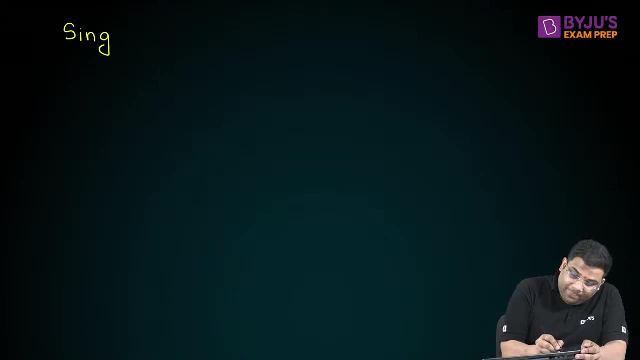 What This is: single pile, A single pile in a single layer Right. This is a single pile in single layer Right. There were no multi layers, But it is quite a possibility that the pile might be driven into a multi layered clay. 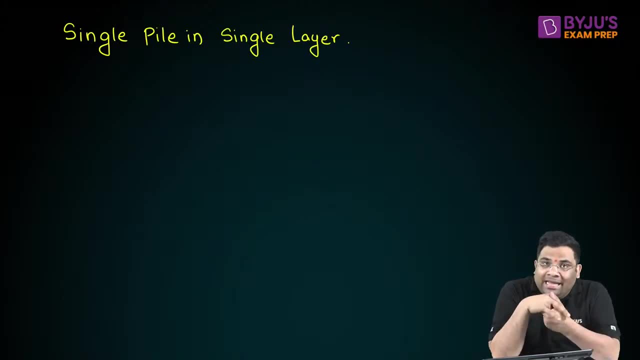 If it is driven into multi layered clay for different layers, what will change? The alpha might be different, The cohesion might be different, Right, So let us see that particular case. Okay, So next thing is what we will study. 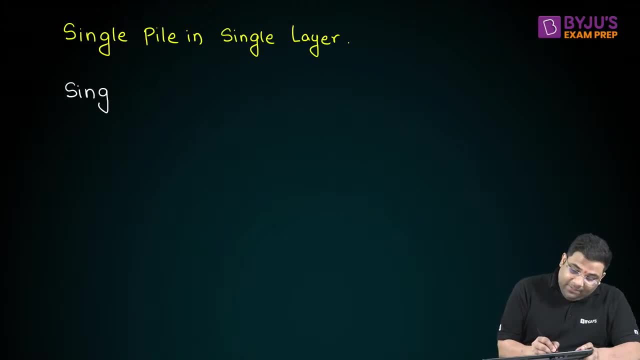 Next thing we will study is a single pile, A single pile in multi layer. A single pile in multi layer. Let us understand this interesting thing: Single pile in multi layer, You see? Okay, This is a single pile in, Okay. 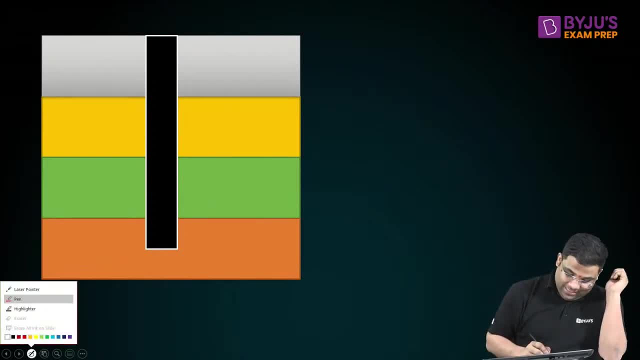 Multi layer. Okay, Now, in this case, how to solve the cohesion. I will tell you the understanding. It is very easy actually. You see this is a single pile And suppose this is the ultimate load. Isn't the pile looking beautiful? 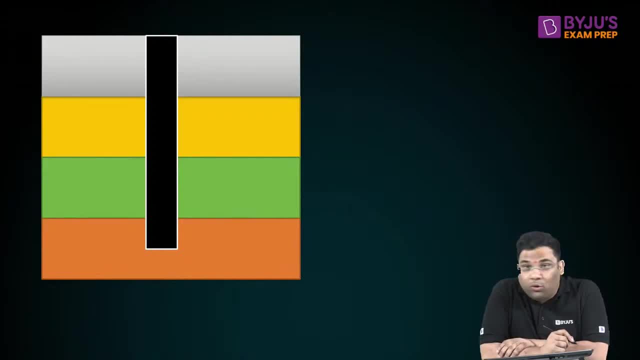 The pile is looking beautiful, or the layers are looking beautiful, Or the whole projection is looking beautiful. I think everything is looking beautiful, Right? So this is suppose the ultimate load. Suppose this is your ultimate load. Okay, Q U Okay. 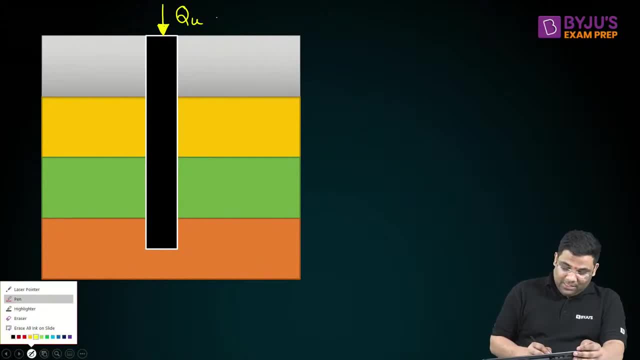 Now, this particular layer, this particular layer or multi layer of clay- suppose the total length is something- But in the layer 1, only this portion of the pile is there. So only this much matters. Okay, Only this much matters. 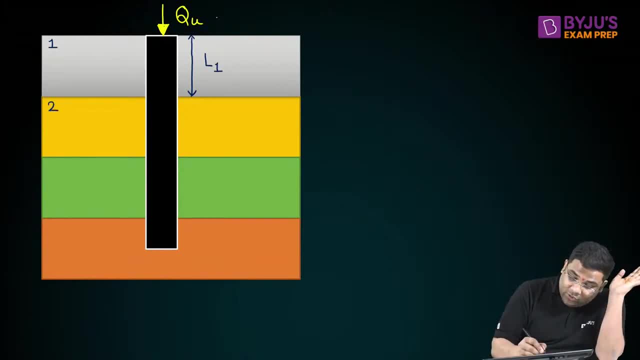 And L1 for the layer 1.. Similarly for the layer 2,. only this much matters: L2. Right, And for the layer 3, this L3. And for the layer 4, I have to take only till where. 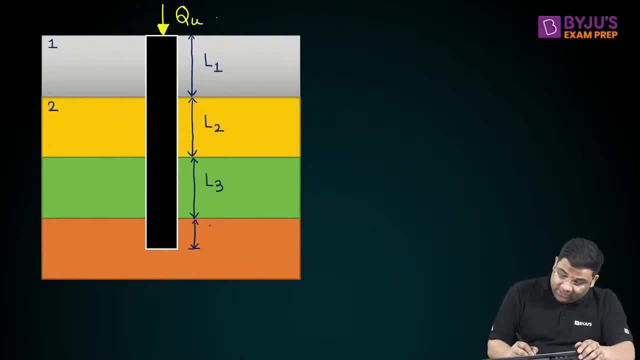 Only till where pile exists. So it is what It is: your L4. Understood. So you have to divide the length of the pile into individual length And be careful about The last layer. In the last layer, you will not take the total depth of the layer. 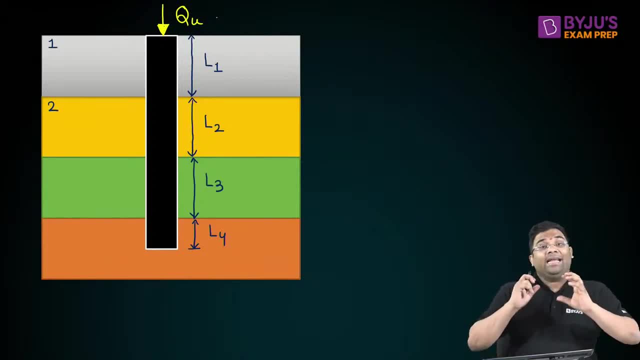 You will take only that much, which is there attached to the pile. Okay, Now you see, this is the third, second layer. This is the third layer. So here I am doing four layers. In the examination it might be two layers or three layers or even five layers. 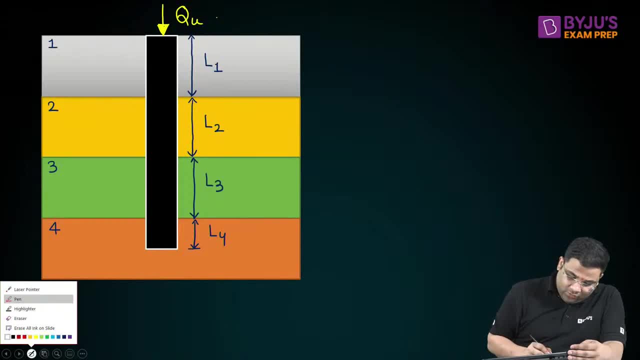 It does not matter, The concept will remain same. So you see, the alphas will be different. Right Here we will have alpha 1. And then cohesion 1.. Here will be alpha 2., Then cohesion 2.. 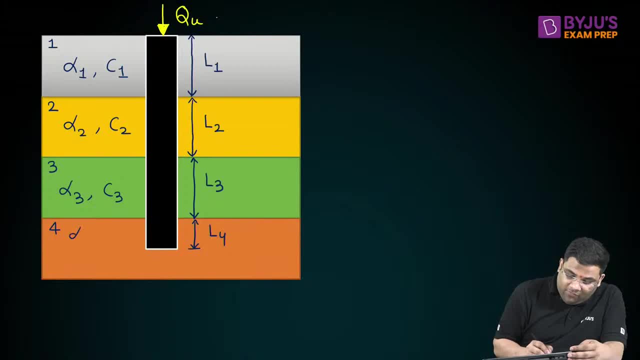 Alpha 3. Cohesion 3. Alpha 4. And cohesion 4. The alpha and the cohesion will be different. Now see when I am finding this friction resistance. Friction resistance is what The frictional stress into what. 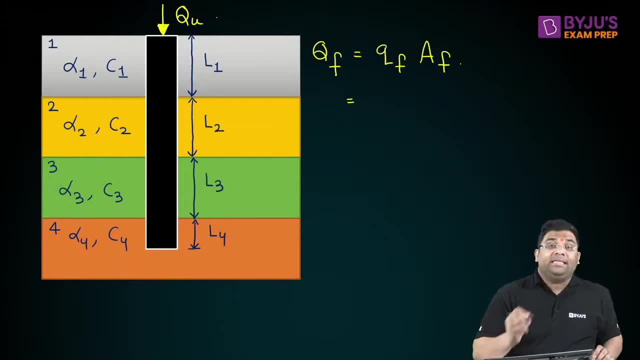 Your frictional area. Now the frictional stress is what? Alpha into C? So it will be alpha into C. Now what is the frictional stress? It is not area, It is surface area. You see, if you see the diameter here, or diameter here, or diameter here, or diameter here, 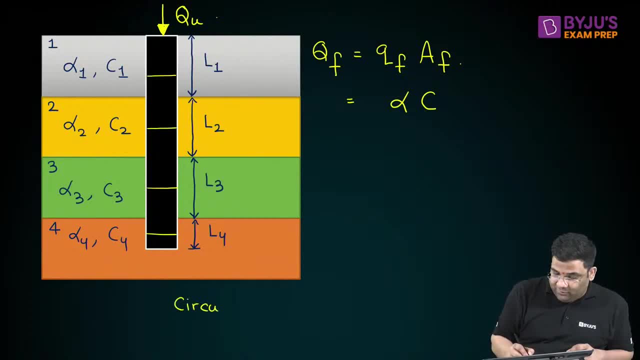 Suppose it is a circular pile. Suppose I am taking this as a circular pile. If it is a circular pile, the diameter is constant. Right, The diameter is constant. Diameter is not changing across the layers, So I can say pi d. 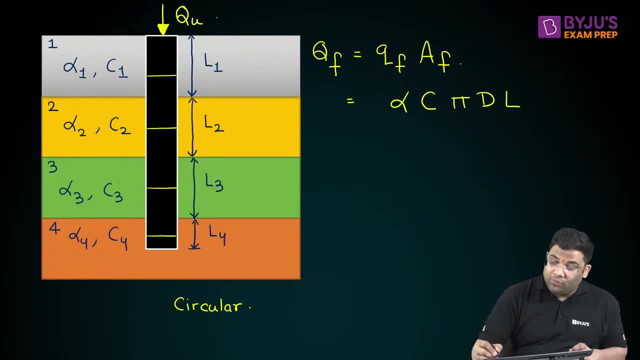 Into what? Into your length? Now you see, We have to take this for different layers. now, Yes, For the first layer, I can say it will be alpha 1, C1.. D will be same, So L1.. 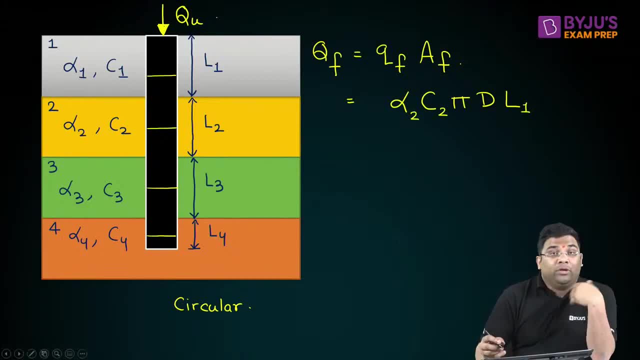 For the second layer it will be what Alpha 2, C2. D will be same L2. So can I say I can take this alpha d common And if you are interested in finding out the total friction. 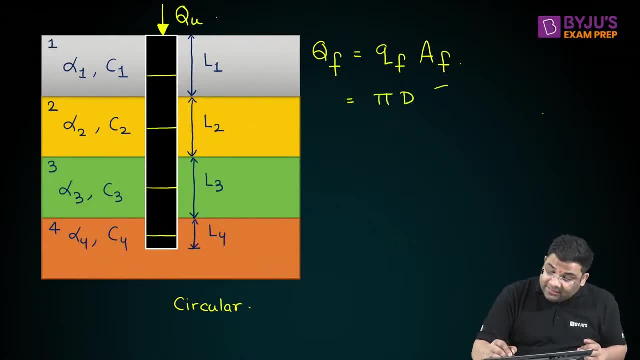 Frictional resistance. It will be pi into d. Summation of alpha i, C, i and then L i: Yes or no, Yes or no. Alpha d C i into L i, Where this alpha d is nothing but the perimeter of the pile. 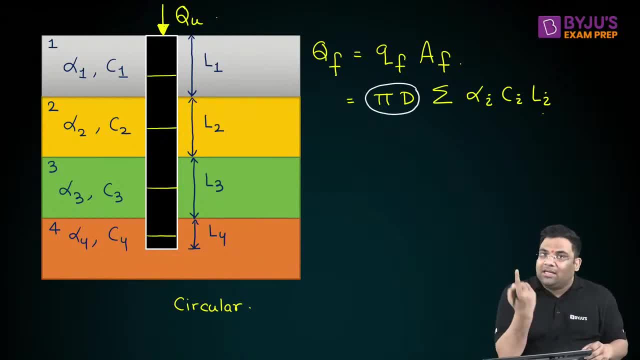 Alpha d is the perimeter. If the pile is circular, alpha d is the perimeter. So here I can write down what Perimeter. So this is the formula to find out. Very simple, right Perimeter into summation of alpha C and L. 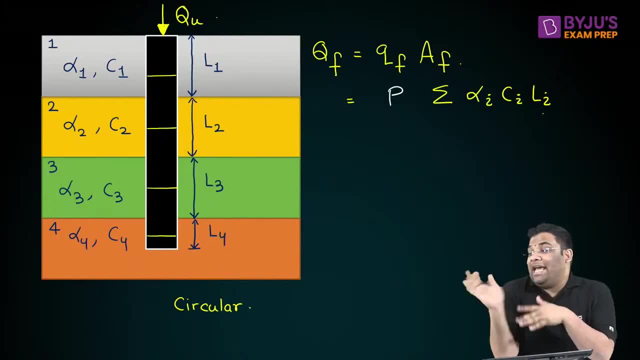 Because, if you see, the different layers, Alpha C and L, are only varying. Only alpha C and L are varying. Very good, Okay, I will say something You know. it will be little difficult to understand. Some smart students can understand. 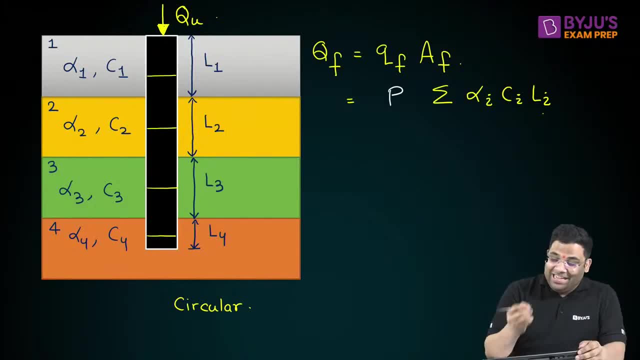 You know, in the diamond. So people are less Okay. Next, let us continue with the class. Okay. Next is QB. Now, what is QB? QB is the base resistance. What is your QB? QB is your base resistance. 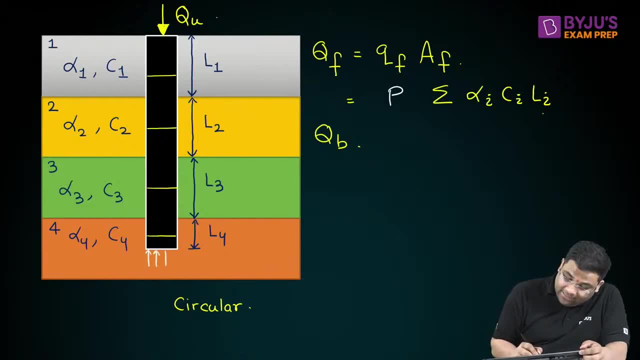 Now see, Base resistance will be here right. Base resistance will be here Now. if I am taking the base resistance, I will take 9 into C Right And then the area of the base. Okay, Area of the base. 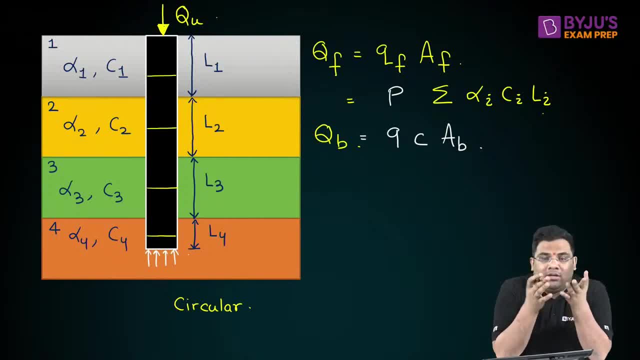 The area of the base will depend on what. It will depend on: circular or square. Now, this C, which one I will take. Tell me Which C I will take here. Tell me Which C I will take. Which C I will take. 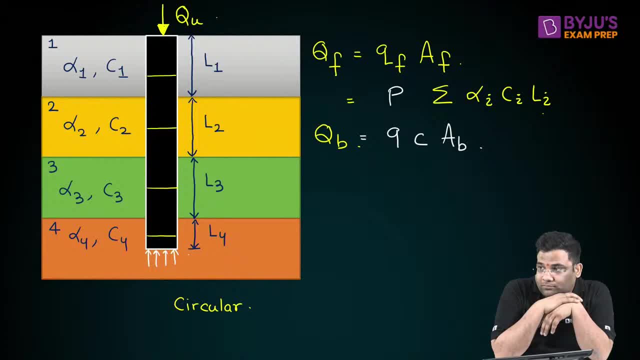 C1, C2, C3 or C4? C1, C2, C3 or C4? Which C? I will take C4. Or I can say the cohesion at the base, Or I can say what I can say: the cohesion at base. 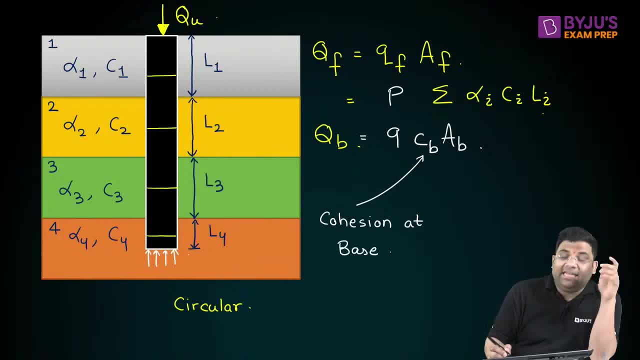 The cohesion at base. See, if it was 3 layers, then C3.. If it was 2 layers, then C2.. So I am going to tell what Cohesion at base. Now, no need To remember this formula, understand this. 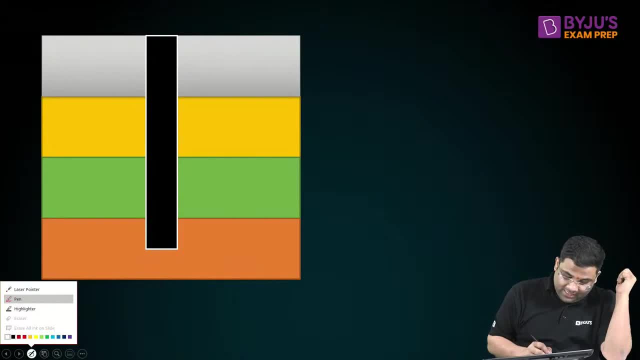 Simply understand this, Suppose I am telling that this individual layer of thickness, you know, suppose I am telling: first one is 2 meter, second, one is 3 meter. third, one is 2.5 meter, fourth one is 4 meter. 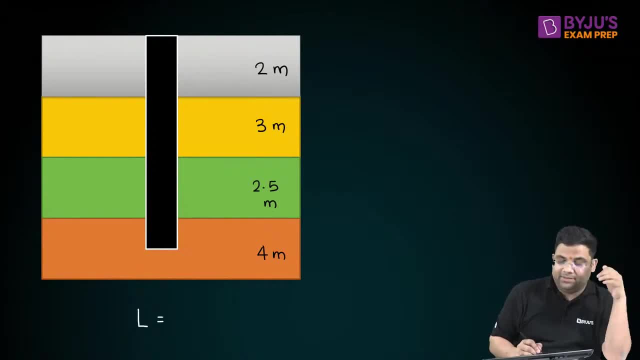 Okay, And the length of the pile is given as 9 meter. The length of the pile is given how much, It is given 9. 9 meter suppose. And then I am saying that for the first layer the alpha is 0.6.. 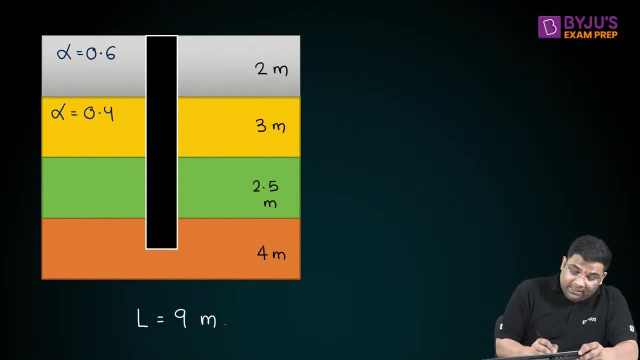 Second layer alpha is 0.4.. Third layer alpha is 0.7.. And the fifth layer alpha is 0.5.. And the cohesion values are 30 kilopascal. Okay, Then 40 kilopascal, Okay. 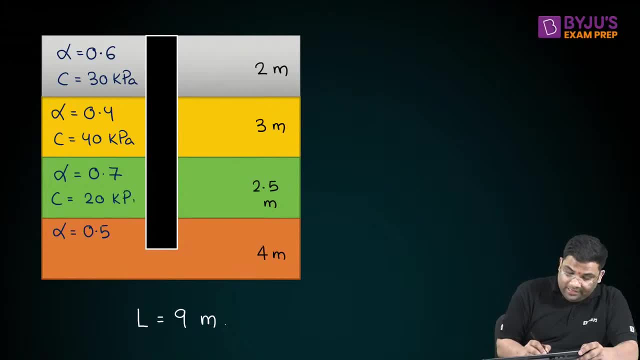 Then 20 kilopascal And then again, suppose, 50 kilopascal. So these are the different cohesions and your different lengths. Smart, after all. Okay Now, first of all, if I ask you find out the frictional resistance, please first give me. 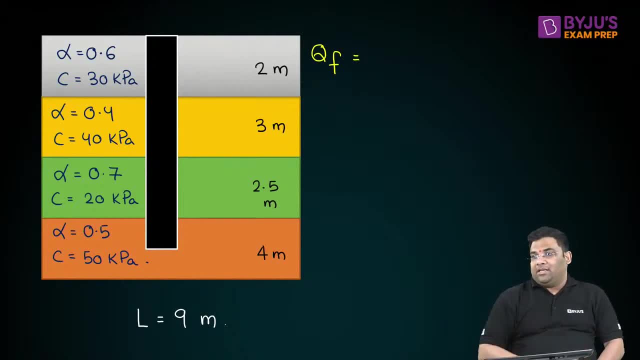 the frictional resistance First, give me the frictional resistance, only I will give you some time. I will drink again Some water. Okay, Find out the frictional resistance. Find out the frictional resistance, Do whatever you want, Do it. 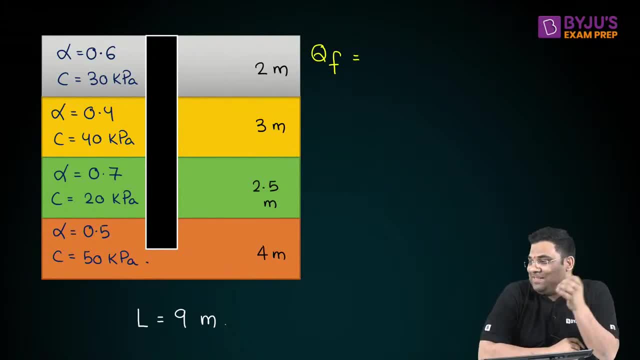 And now focus up on the class. Please find out the frictional resistance. Okay, This method you have understood. Oh, diameter, Oh sorry, sorry, sorry, Very good, Karthik, Sorry, It's a square pile. 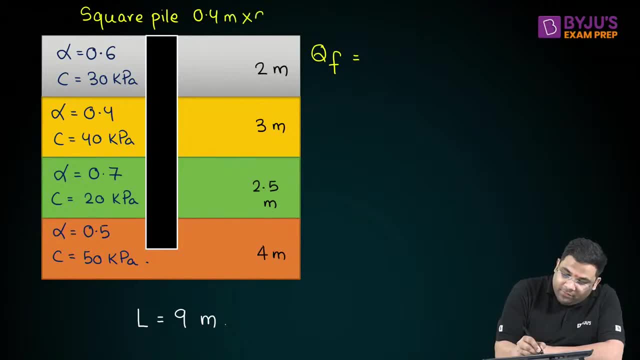 0.4 meter into 0.4.. 0.4 meter into 0.4.. It's a square pile, okay, Sorry, sorry, Square pile, Square pile, Square pile. Very good, Smart and fast, That's good, It's very easy. First of all, it will be what I told perimeter into summation of AI. Last letter is 4 meter: AI, alpha, alpha, alpha, I, then CI and then what Your LI. 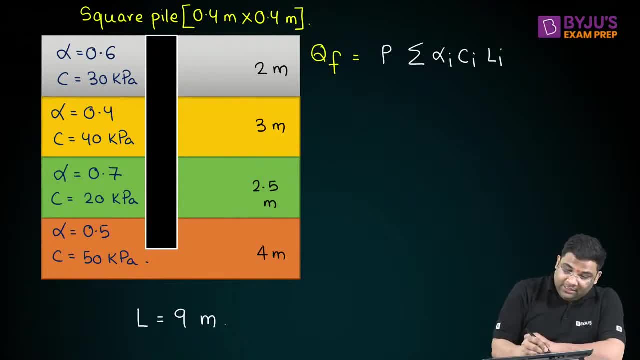 Okay, You see, for the first one, this length will be equal to how much? 2 meter only. This length will be equal to 2 meter only. This length will be equal to 3 meter only This length will be equal to 2.5.. But for the last layer, I will take how much? Tell me How much L4 I will take. Tell me How much L4 I will take. Please mention in the comment section How much L4 I will take, How much L4 I will take. 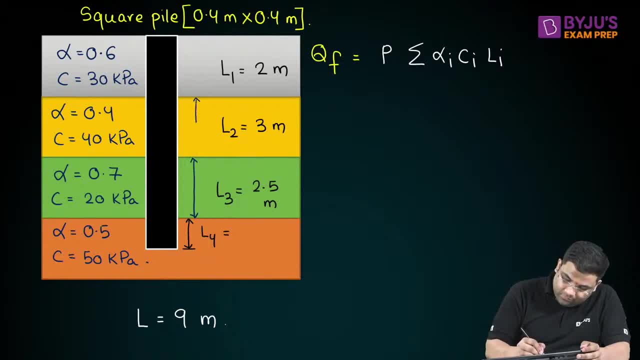 How much L4 I will take. Yes, Very good, Because the total length is given as 9 meter. The total length is given as 9 meter, You see. So this length will be what 9 minus 2 minus 3.. 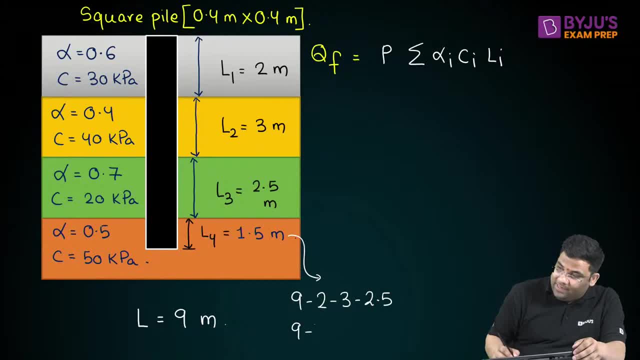 3 minus 2.5.. That is 9 minus 7.5, giving me how much 1.5.. Understood from the diagram, Simple, from the diagram you can find out. Now the game is over. Now the game is over. So the perimeter, it's a square pile Perimeter will be 4 into side length, right? Yes, So 0.4 into 4, it is 1.6.. It will be 1.6.. And for the first layer, 0.6 into 30, into 2.. 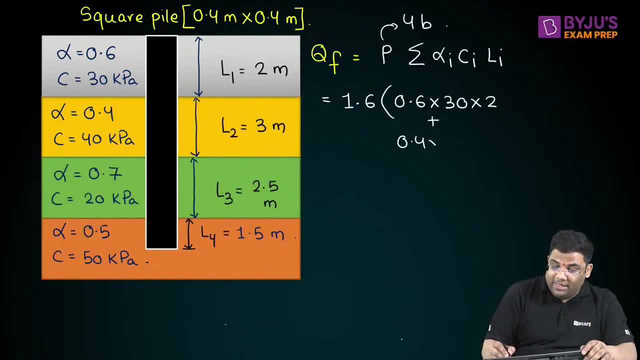 Right, For the second one it will be 0.4 into 40 into 3.. So this one, last third one, 0.7 into 20, into 2.5. Right, And for the last one it is 0.5 into 50, into 1.5. Yes, So QF, if I ask you just find out the QF, it will be equal to 1.6 into the first layer, Right. 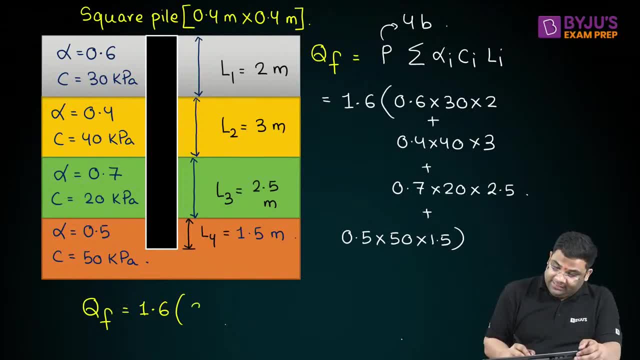 First one is 18 into 2.. That is 36.. Second one is 16 into 3.. 48.. Then it is 50 into 0.7.. 35.. And last one is 25 into 37.5.. Okay, So many are getting this answer, So the answer is: how much? 250.4.. 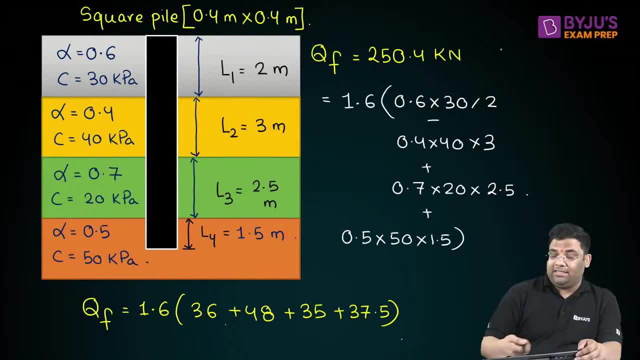 You see how just by simple understanding of the things You can find out these answers. No need to be having what Too much of complications. Very simple, Okay. Somebody wrote the answer: 11.83. now Okay, So welcome to the class. Something happened, Okay. 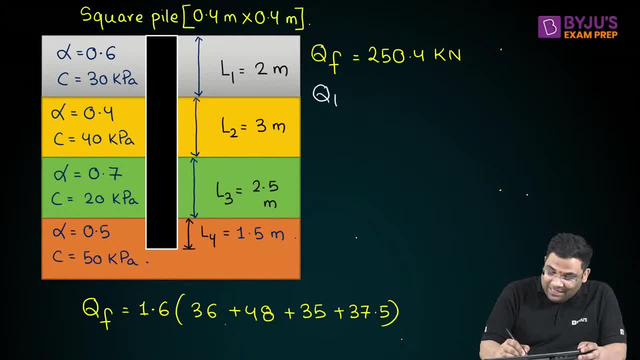 Next is your base resistance. Now, base resistance is very simple: 9 into the base area, Not base area, Base cohesion. Base cohesion is this: Right, 50. Right. So, 9 into 50 into the base area will be how much B square? 0.4 square. 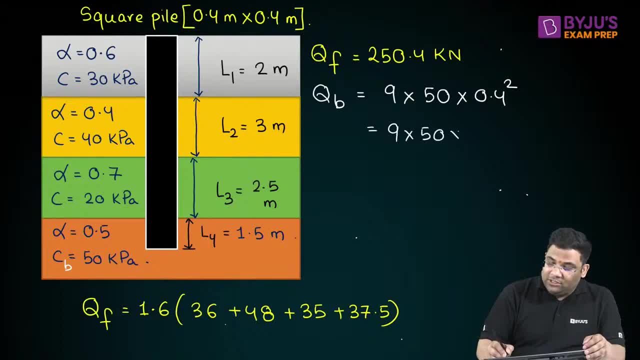 That is equal to 9 into 50, into this will be 0.16.. So how much you are getting this? 1.6 into 5.. 72.. Right, I think 72. you are getting Base resistance Right. 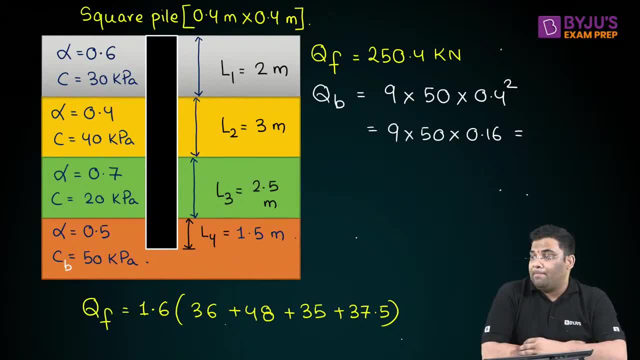 Getting how much? 72.. Right, How much. you are getting Base resistance: 72 kilo Newton. You are getting 72 kilo Newton. So this is your base resistance, This is your frictional resistance. So total ultimate load will be equal to how much? Just add this two, It will be 322.4 kilo Newton. Okay, 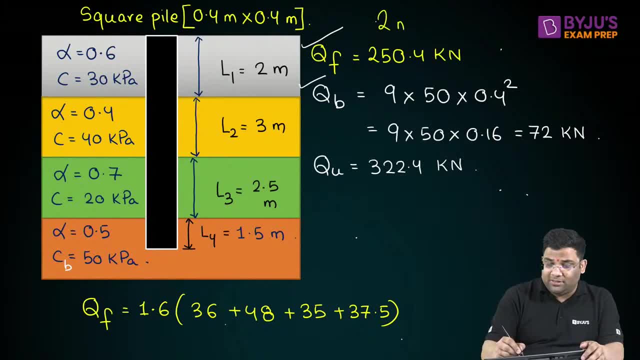 So you see, so nicely, You see two more questions, Suppose in the examination, in the gate examination, and suppose the same question can be asked, as the same question can be asked as your SSCJE mains question. SSCJE mains question. Okay, SSCJE mains. Suppose they will ask you 15 marks or 20 marks. 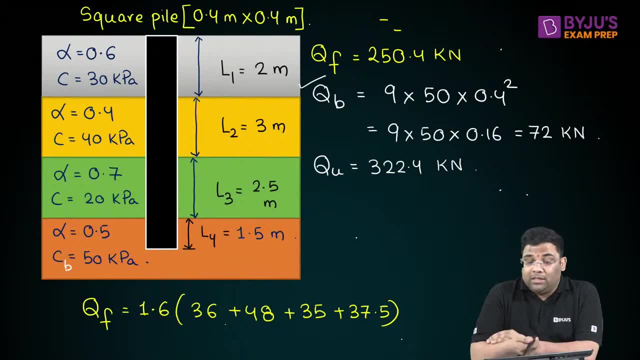 Okay, You should prepare for both. You should prepare for both: SSCJE plus gate. You should prepare for both. Actually, if you are preparing for gate, see, I will just give some time here. Okay, So this is the end of the question. 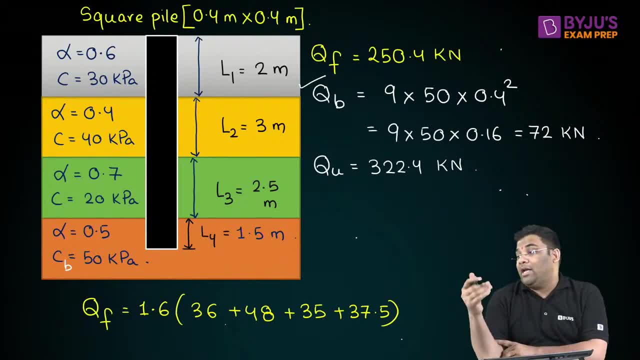 Please answer that. Are you understood? You understood this question or not? Then I will answer Pravin's question also. So this we solved? Yes, And we saw that two type of things we saw- Single clay, single pile in a single layer. 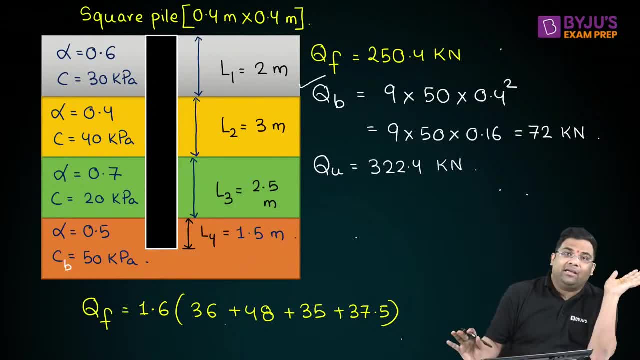 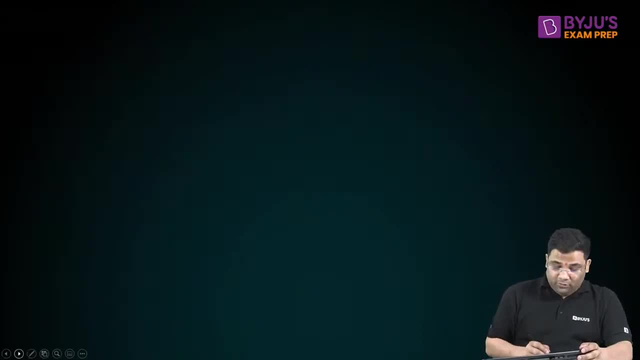 And then we saw single pile in a multi-layer. Okay, Single pile in single layer, Then single pile in multi-layer, Very good. Now, coming to Pravin's question that he is asking that sir, should I prepare for SSCJE plus gate? 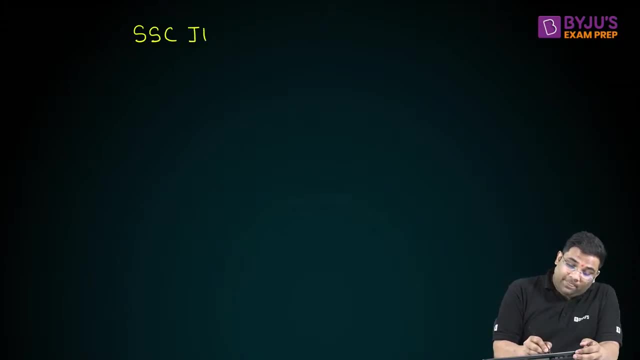 See, I will tell you. I have told before also: SSCJE has two stages. One is your prelims, One is your gate. Okay, Sorry, your ESC mains, SSCJE mains, Okay, Okay, Your prelims. SSCJE prelims is gate one marks. 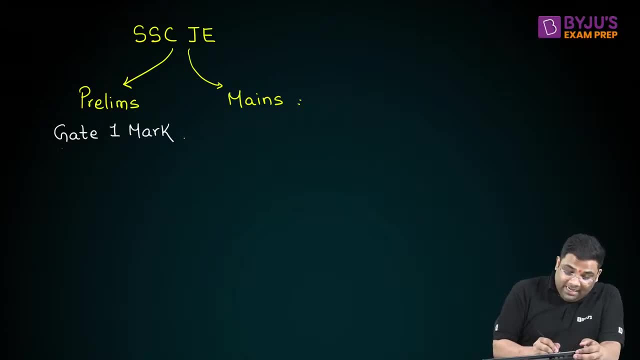 It is prelims: one mark: Okay, The gate: one mark, as asked in the prelims: Okay, And your gate two mark questions: Okay, Gate two mark. questions are asked in what: Your mains, Okay, Your mains. 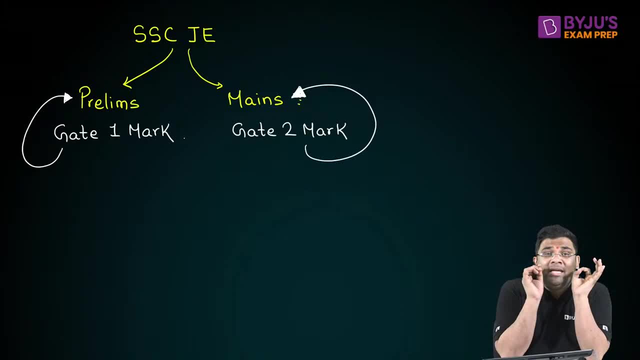 Okay, Okay. So, if you have, you are preparing for gate. indirectly, you are preparing for what Your SSCJE. Indirectly, you are preparing for what Your SSCJE. You just need to study what Your aptitude. 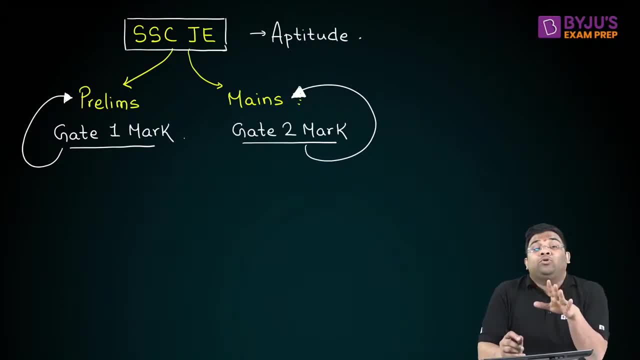 Yes, your aptitude Okay, And aptitude also, the syllabus is similar And some additional GS And some additional GS. So, Mr Pravin, if you are preparing, if you are preparing for gate, indirectly you are preparing for SSCJE, with a minor addition of GS. 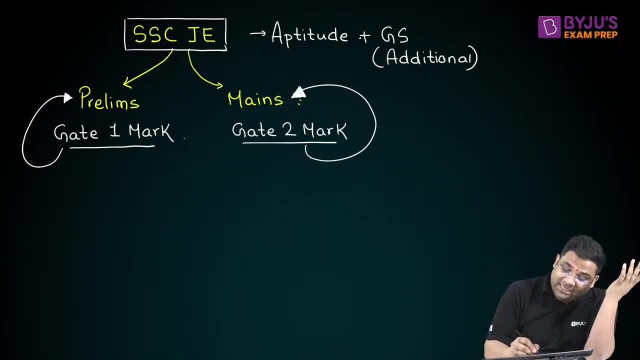 That's it, The minor addition of GS, Because you see, this aptitude also is common. to gate, It is also common to gate. So that means your aptitude and then your prelims questions and then your mains questions. all these things are common. 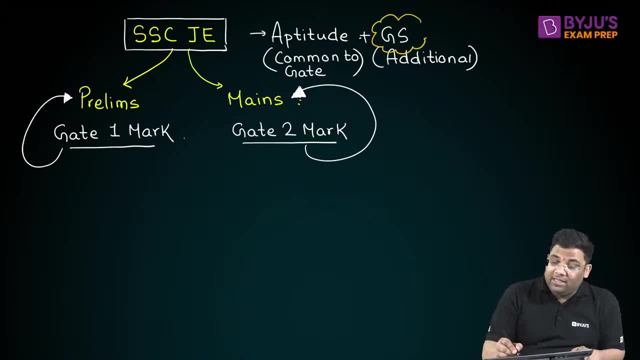 So additional thing is only this: GS. Okay, So I have taken a complete lecture on how to have a combined approach for gate and SSCJE. I'll request someone to put that link in the comment section. Okay, Some student can put the link. 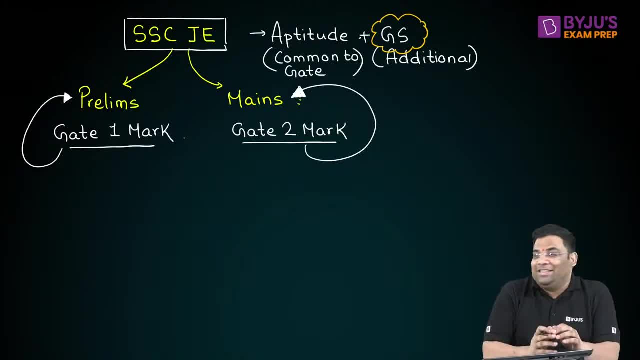 Because I don't have the method to put the link in the comment section. You can put the link in the comment section. And, Pravin, if you have seen that lecture, very good. If you have not seen, then you can go through that. 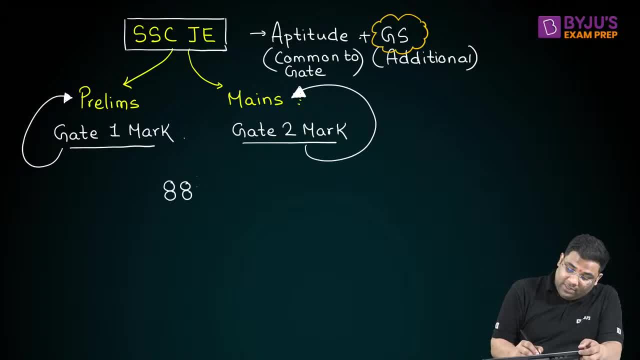 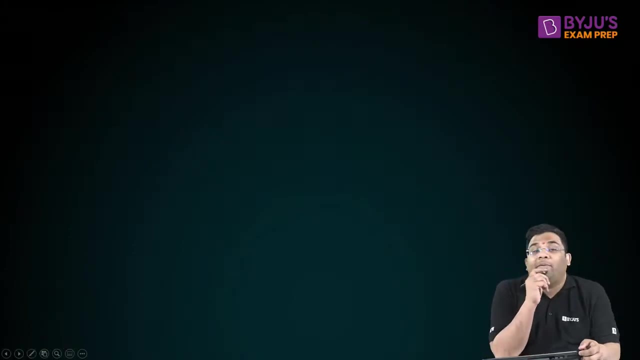 If you have any other doubts or you still are confused or you want any other clarification, then you can message me on my number and you can ask me your particular specific thing also. Okay, Thank you very much. Okay, So this was a short inquiry by Mr Pravin. 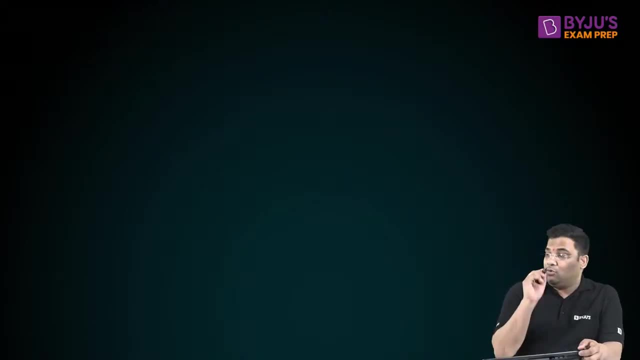 and I hope that I have answered him properly. Now let us go to the next thing. The next thing is what Your group pile. The next thing we study is what Your group pile in clay. Now the group pile in clay. 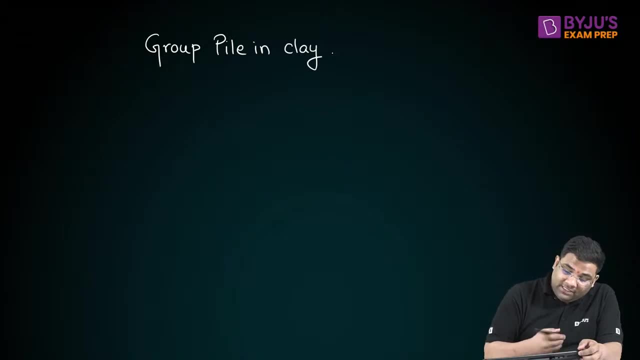 How to find out the group pile Now. how to study the group pile. Okay, Now in group pile they will also ask the ultimate load capacity, not of the pile, but the group. Ultimate load capacity, Not of the pile, but the group. 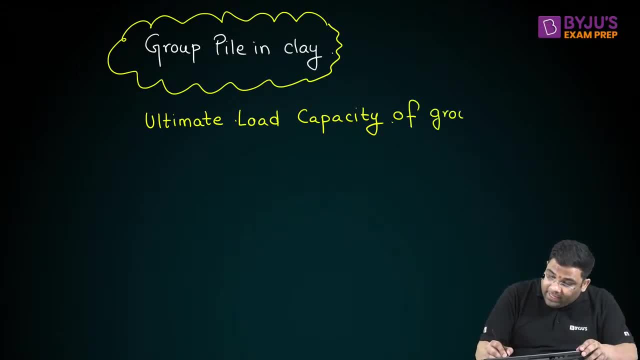 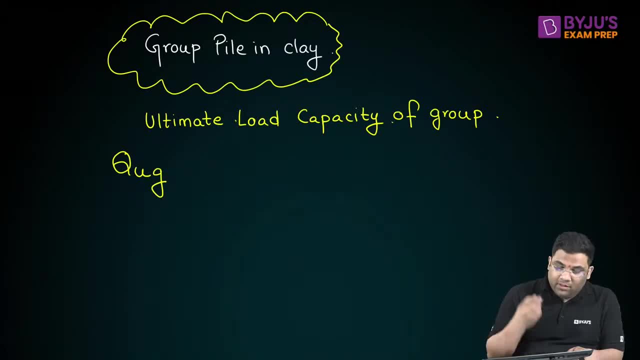 QUG. QUG Means what Ultimate load capacity of the group. Okay, Now you can find out this in two ways, Two ways How The first A is: you assume that all the A piles in the group. they are failing individually. So I will call that as what Your individual. 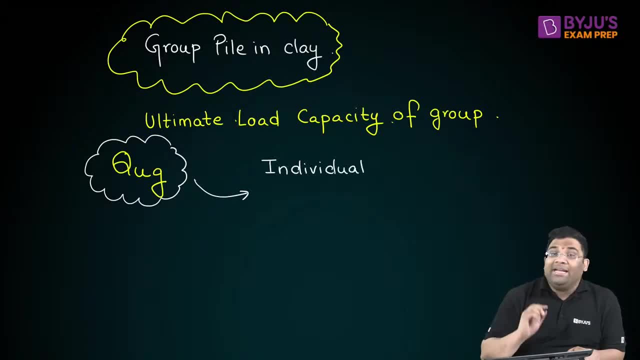 failures. I will call that as what? Your individual failures. If all the piles are failing individually, then I can say that that group, that load capacity of group, is coming from individual failures. I will give the name: what I Q, U, G, Y. Ultimate load capacity of the group. 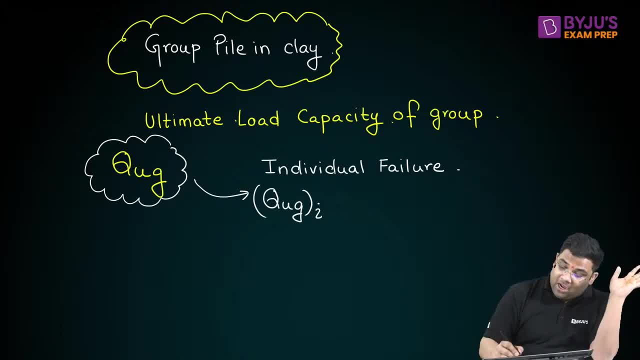 under individual failure. How to find out that? Very easy. If you know the ultimate load of each pile, then just multiply into the number of piles. That will give you what The ultimate load capacity of the group under individual failure. Individual failure means what. I am, assuming that all the piles are failing individually. 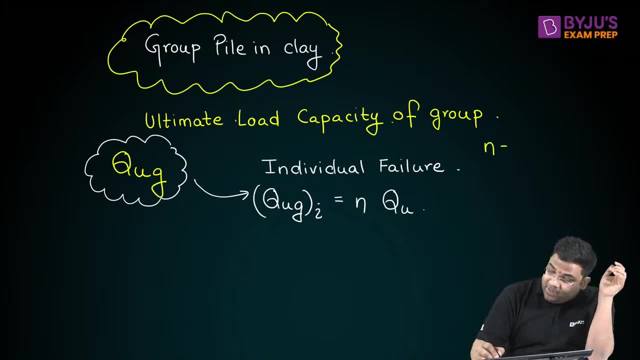 Very good Where. N is what Your number of piles. N is what Your number of piles. Now the next thing? The next thing is: what is the next thing? The next thing is: I am assuming now that piles fail in a block, Piles fail in block Means together they fail Together. 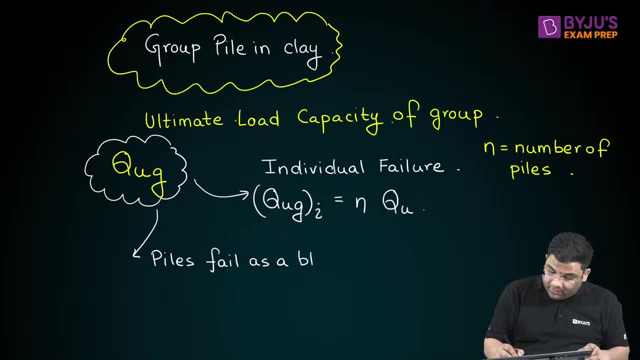 they fail, Fail as a block, Together they will fail, And that I will call as what? Q U, G And failure is what As a block? How to find out this? I will explain now, Don't worry, I will explain now. See, this one was pretty simple, like individual failure, right? 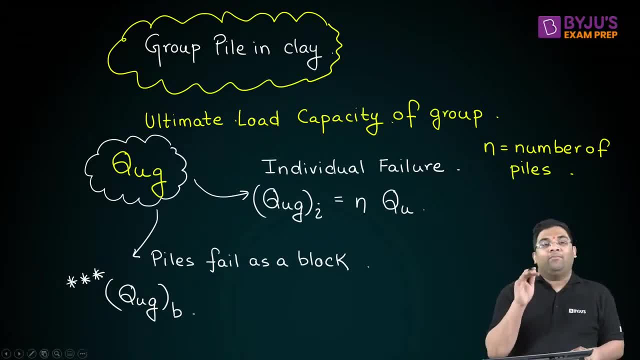 So individual failure is very simple, That for one pile it is this much, For N piles it will be this much. Very easy. So individual failure was easy. Second one is when they fail as a block. So when they fail as a block, then how to find? 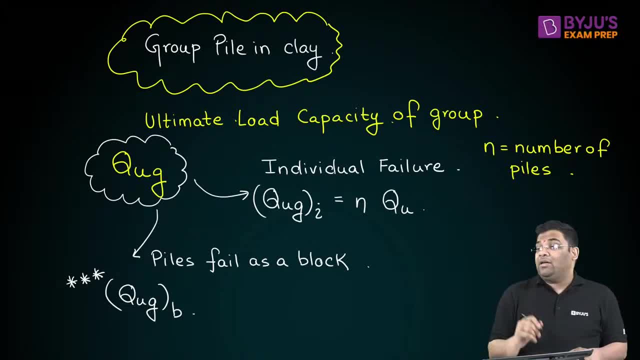 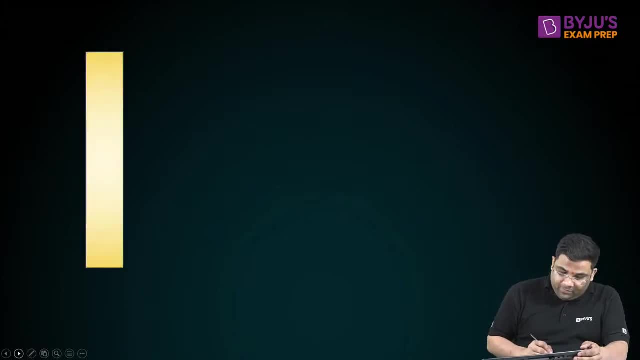 out. Let us see. Let us see Very easy: Understand the concept. don't remember it. If you understand concept, you will easily able to solve. Now see, this is single pile. Now, this single pile, when arranged in rows and columns, will give me a group pile Something like this: 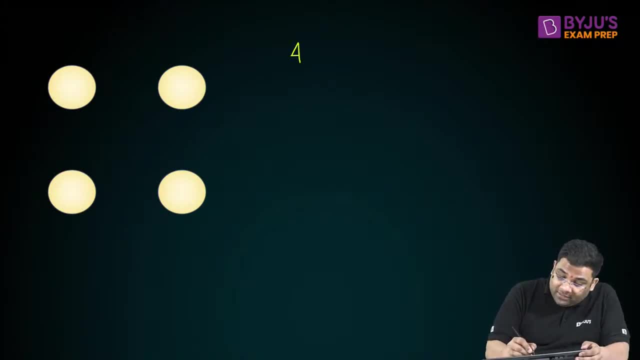 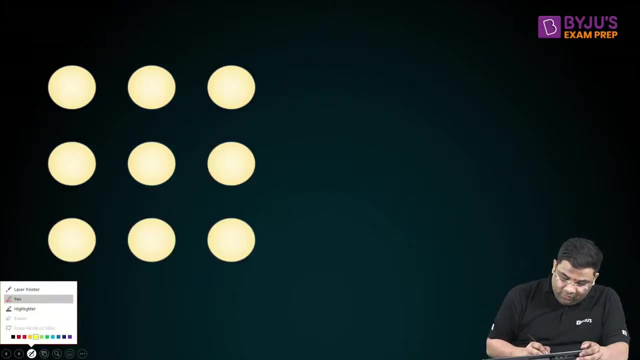 Suppose this is what. This is a group of four piles. So group of what? Four piles, Okay, And this is forming a what? It is forming a group pile. So I can say here: N is what Four. Now let us see the next example. It is what? 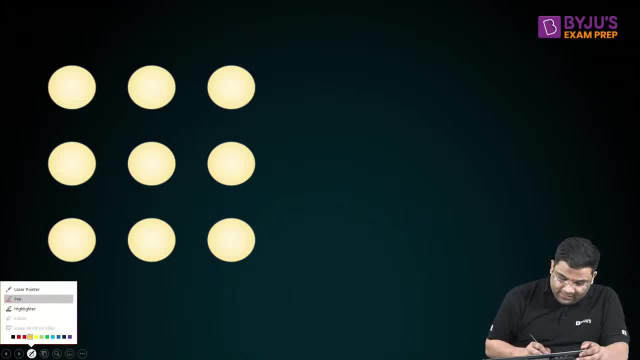 Your nine piles. Yes, Here, what N is your nine. So group of nine piles. So now you see this group of nine piles and they are failing as a block. So you see this. Are you able to see the block? The block is a square right. You see, the block is a square na. 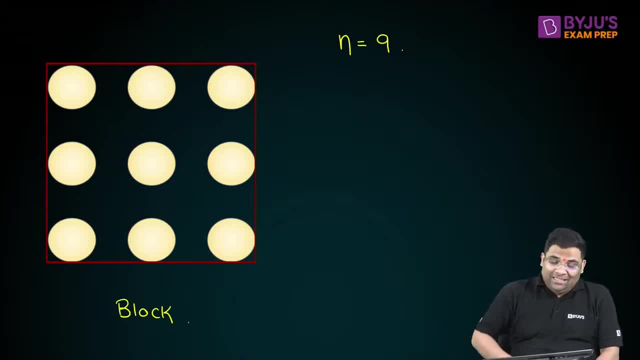 You see the block is a square. na. Yes, And suppose this centre to centre distance, Suppose this centre to centre distance is S. This centre to centre distance is S is S. You see, this will be D by 2, right. 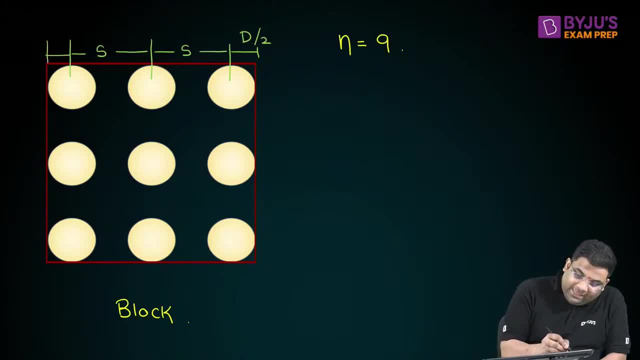 And this will be d by 2.. So I can say, if they are failing as a block, they are failing as a single block, then they are forming actually a square. They are forming actually a square and I will call this as width of that particular square. capital B right. 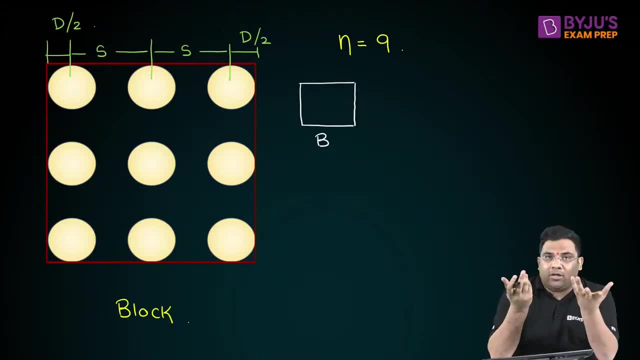 Right Width of that particular square, or I can say block width of the block right. It is the width of the block right. And now this width of the block here in this case was 2s plus d right. It is 2s plus d right. It is 2s plus d. 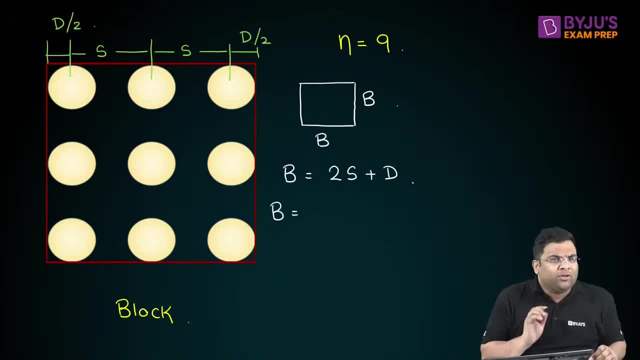 I can write down this actually, as this 2 is actually what It is actually: the r minus 1 into 2s plus d. This 2s is what 2s plus d is what r minus 1 into s plus d. Welcome, Salgar. Now this r is number of rows, right? You see, r is number of rows, or I can say number of columns, right? 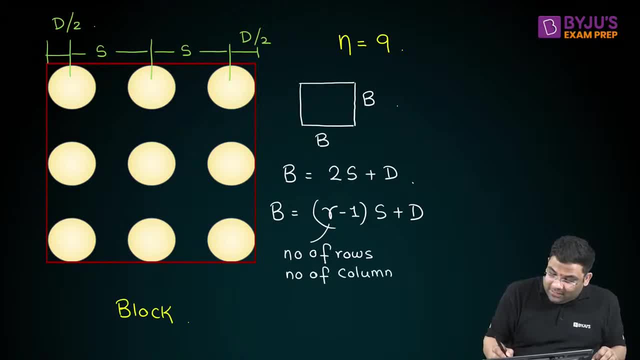 It is the number of rows or the number of columns. yes, Or, if you do not remember this formula, by C, also, you can find out right. Yes, There is no need to remember this formula. There is no need to remember this formula also, Let us forget this formula. okay, Even if you do not know the formula, by seeing are you not able to see or what? Yes, You can see and find out. right, You can use your common sense. 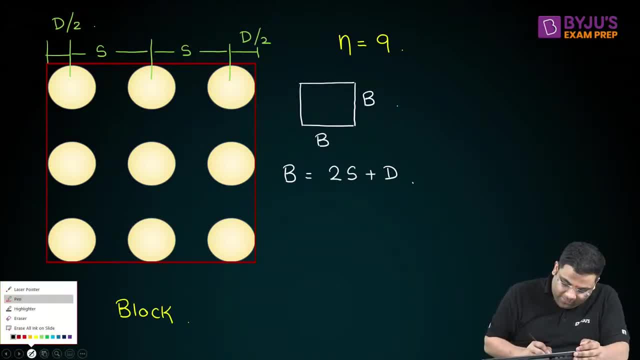 So here, this is what. This is your width of that block, This is the width of block. This is the width of block, And by seeing, only I can find out this width. Now this whole block will act as a single square by line. 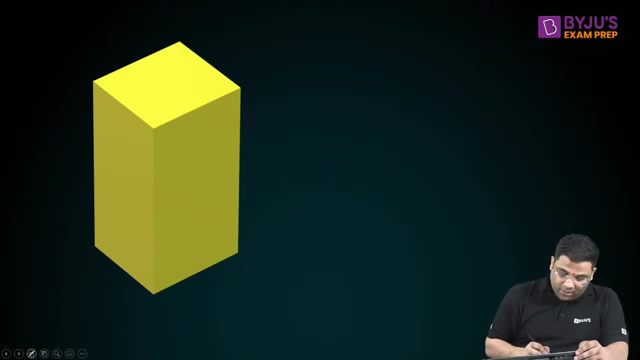 Like this: yes, This whole block will act as a single square pile. yes, Now this has become a block. yes, Now this has become a block and they will act as a single square pile. They will act as a single square pile. Suppose this is what Top view will. this is the 3D view I can say: Are you able to imagine now? 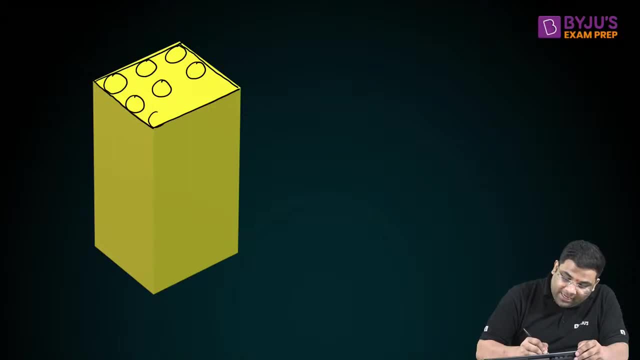 Are you able to imagine now, But how this group pile become a block right? It has now become a block right, A square block, and I can say this is the width of that particular block. So now, if I am considering the block failure, that will be what The ultimate capacity of the group, and I am considering block failure. 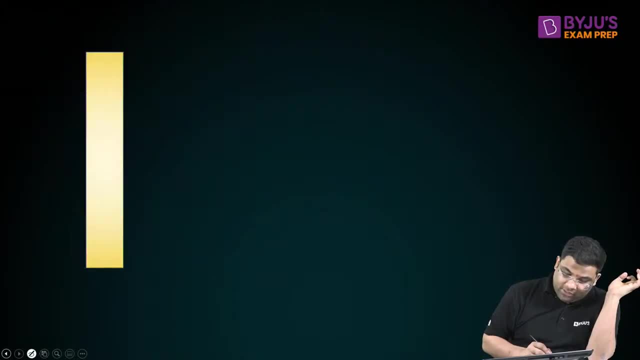 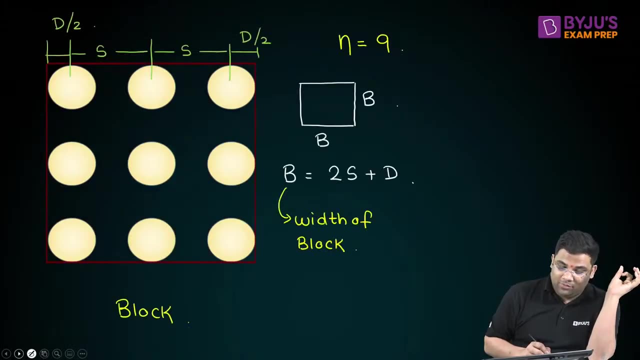 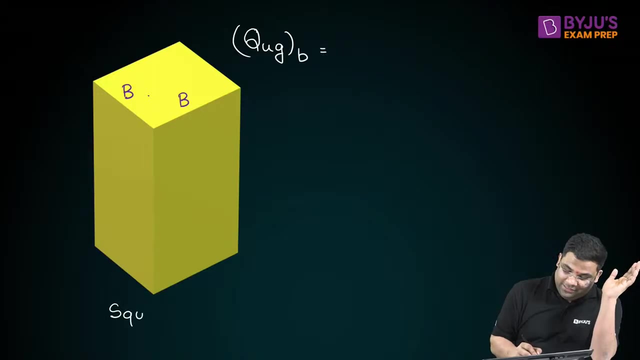 I am considering Block failure. That is what I told you initially: Block failure, right. So now just treat it as a square pile. now, Just treat this as a square pile. Just treat this as a square, big square pile, right. 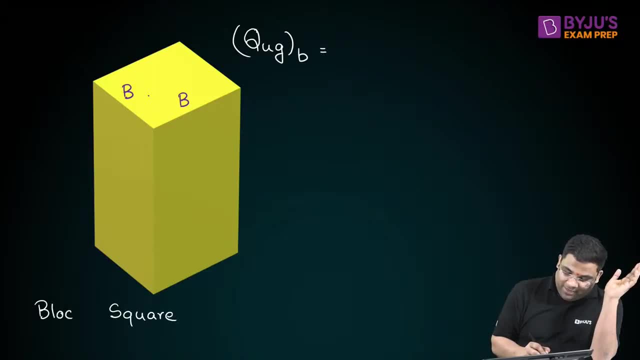 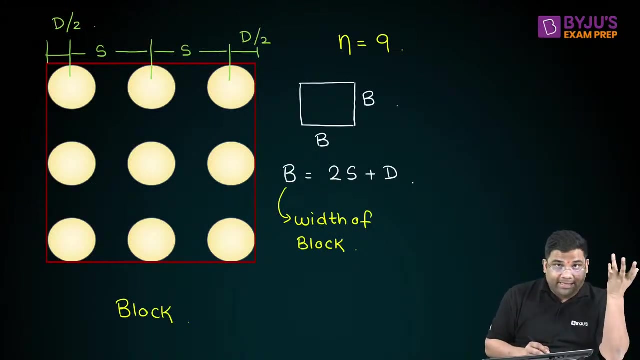 Big this block you consider as what A big square pile right Now, this square pile, this block square pile, will have the same length, right, It will have the same length as that of what Individual piles, Individual piles, Just this side length will be different. And how to find out This side length? I told you width of the block, or side length of the block right, Very easy. 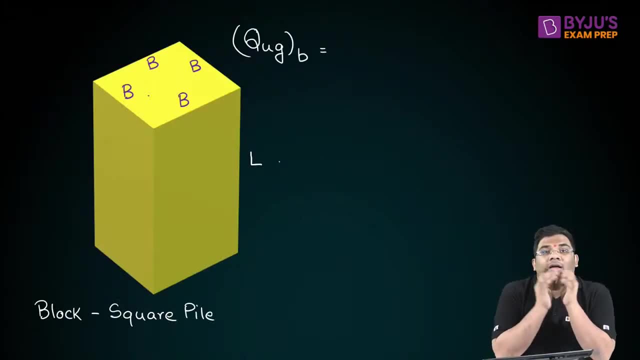 Now what you can do. Apply the formula. It will be what The frictional stress? Frictional stress is what Alpha into C? Then what Then the surface area of the block. Surface area of the block will be how much? 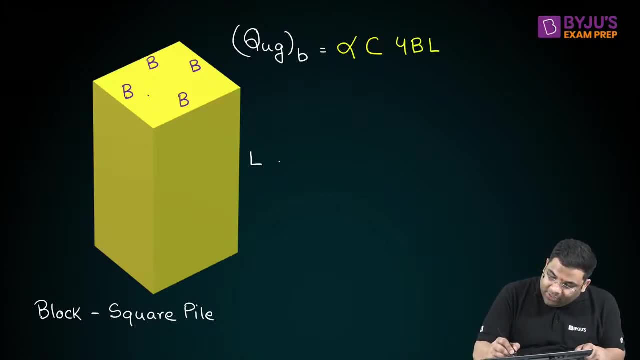 Simply, Simply, Simply Simply: 4 into capital B into L right, 4 into capital B into L. Now it has just become what? Now it has just become what, Tell me. Now it has just become a square pile. 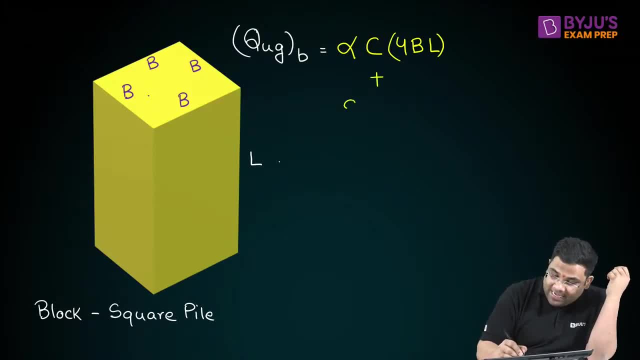 Kutam Plus your 9C, the end bearing resistance into the base area. Base area will be B square. right, Right Base is a square pile. Base area will be how much B square? So so easily you are able to remember the formula for the block failure. No need to remember anything, Just treat it as a square pile. Just treat it as a square pile, with a minor variation. If you remember, when I initially told you the single pile, I told that there will be adhesion. between what? Adhesion between this pile and the clay. Yes, 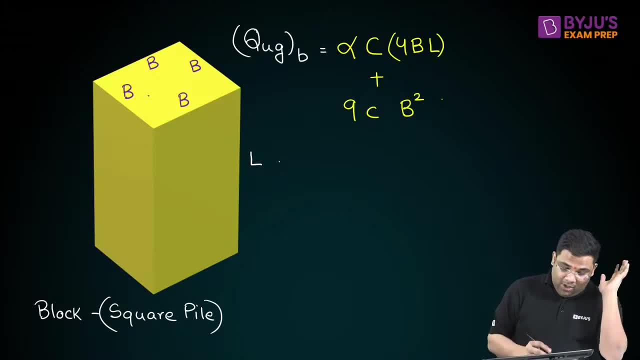 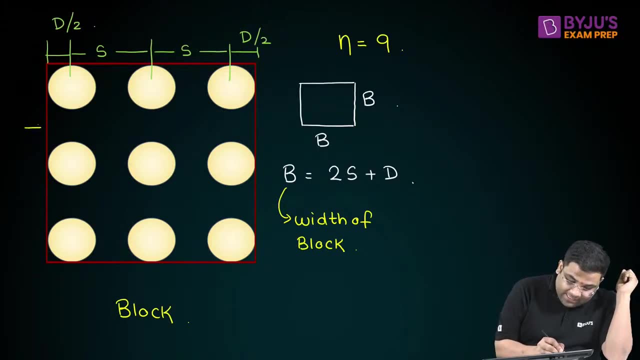 Yes, Pile and the clay, Right Now, here, when it is forming a block, here. you can see, here the interaction is between whom and whom. Tell me When it is forming the block, tell me the interaction is between whom and whom. Clay and clay. Or tell me clay and the pile When it is forming a block, then there is interaction between clay and clay. Or there is interaction between what- The pile and the clay. 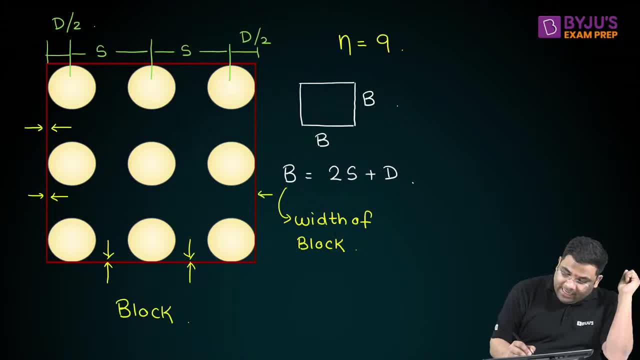 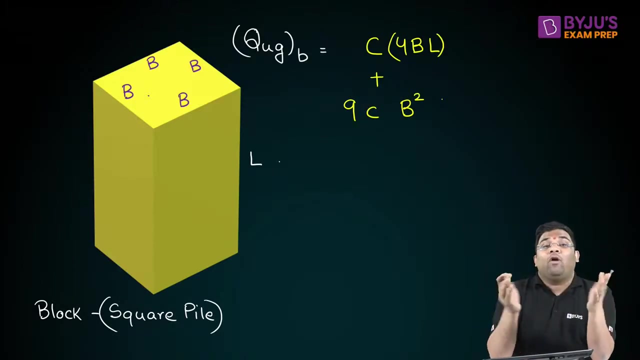 Yes, yes, pile and the clay when it has formed a block. you can say it is having interaction between what Clay and clay, So it is forming a block, So between clay and clay, only your cohesion will be there. or you can say: the adhesion factor is 1, I can say So easy to remember. 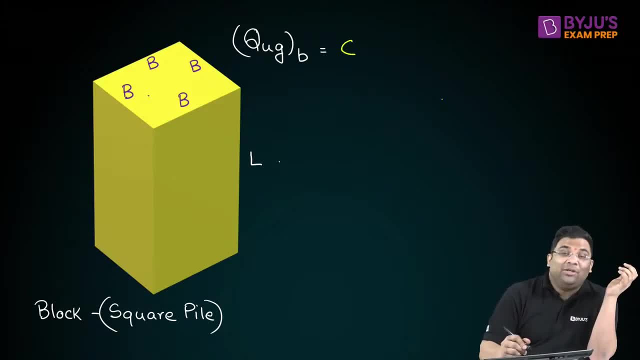 the formula. So I can say this is nothing but C into the surface area 4VL plus 9C into the base area B square So easily you are able to remember. That means, if you know the method to find out the ultimate load capacity, okay for a single pile, you can easily find. 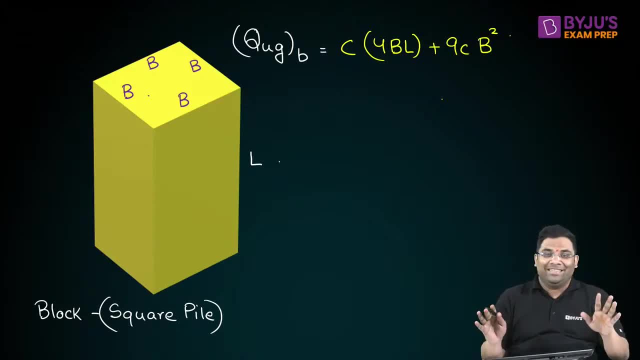 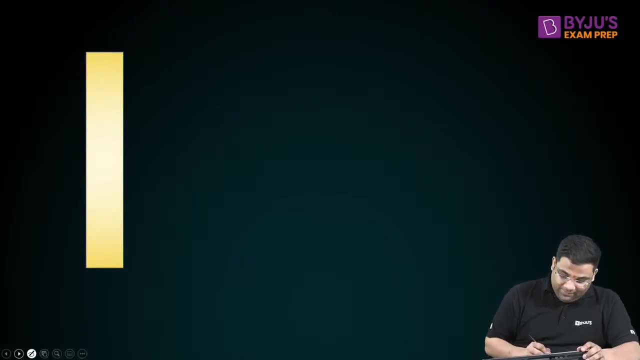 out for a group pile. So easy, Easy. Let us solve one question. Suppose I am giving you that we are having what We are having: similar 9 piles. okay, We are having 9 piles 9.. 9 pile group is there and alpha is 0.6.. The cohesion is 50 kilopascal. okay, Length of. 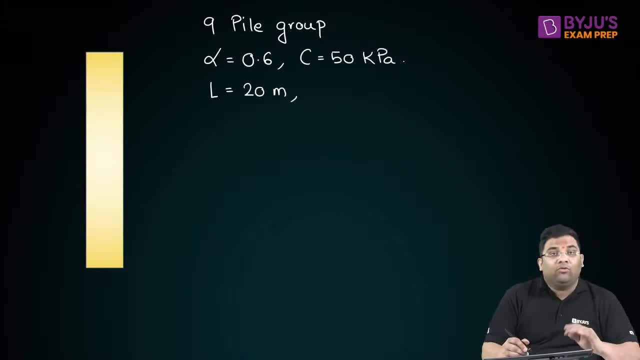 the pile is 20 meter, and suppose they are circular piles, okay. Diameter is 0.4 meter, okay, And spacing between the piles is given, as suppose, 1 meter. I will take 0.3 meter. Sorry, sorry, My health is little down so I stopped. Okay, So now. 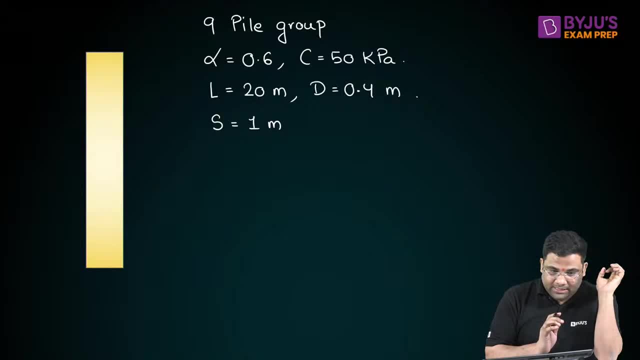 let me make some changes. Alpha C let me take as 40. So the diameter will take 0.4, only length, I will take 20.. Okay, Sorry, My health is really not good. I hope you get the answer. 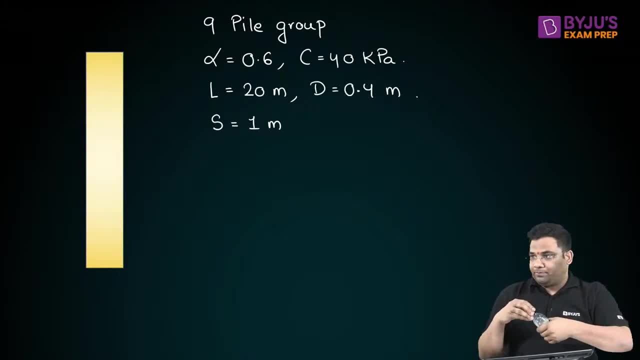 Don't you understand? Sorry, No problem, Sorry, Okay, Thank you. Now, if this data is given, you see, so easily you will be able to find out the group pile capacity. Very easy. First of all, you take what? First of all, you take your number of piles as 9.. 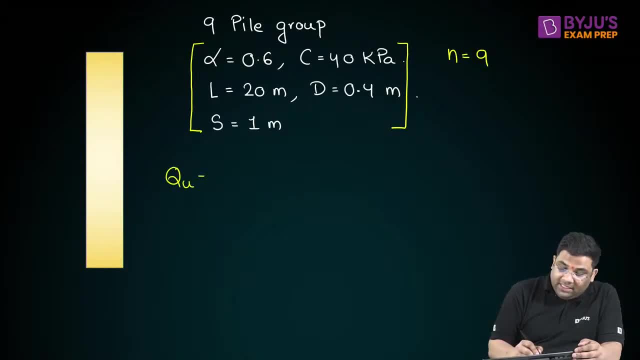 Now for a single pile. you can find out the capacity. It will be alpha into C into the surface area. Now individual pile. take for the individual pile. it will be what Pi D into L individual pile plus 9C into what Pi by 4 D square. 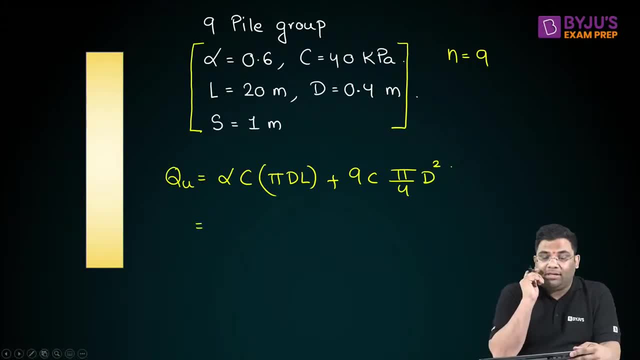 So this: how much you are getting For a single pile? how much you are getting For a single pile? how much you are getting, Tell me? Tell me 810.53.. Okay, That sounds logical. Let me also check a value: 0.6 into 40.. Let us also do 0.6 into 40 into pi. D is 0.4, D into L. Okay, Whatever I am getting, I will add 9 into C into pi by 4.. 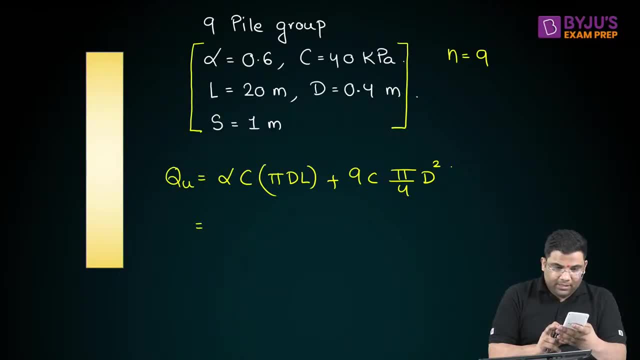 9 into 4, into D square, I am getting 648.1.. Please check, There will be some calculation error. Okay, 648.1 kilonewton. Okay, You have to take here alpha. You have to take here alpha as 0.6.. Why? Because this is individual failure And then I can say the group capacity. when I am considering individual failure, it will be what? 9 into that of a. 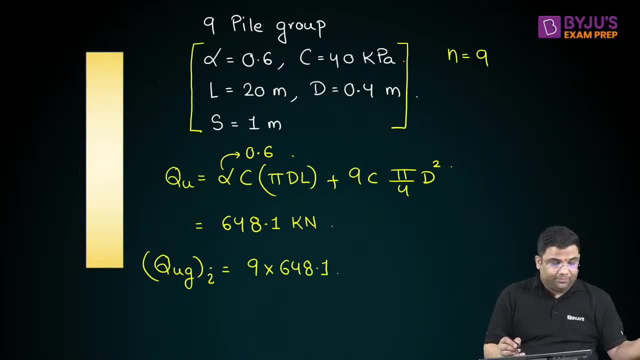 Single pile. So I am getting how much 648.1 into how much Your 9.. I am getting 5832.9.. Okay, This is the ultimate group capacity. when I am considering your individual failure, When I am considering the individual failure, this is: 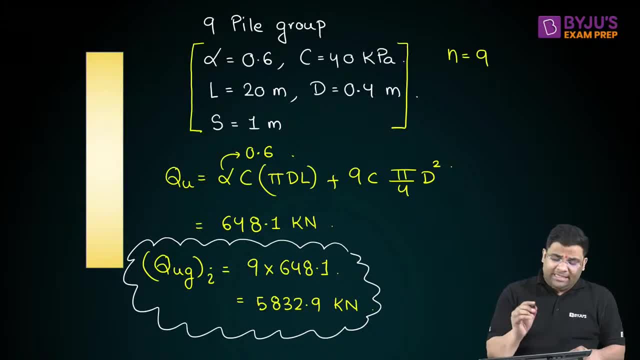 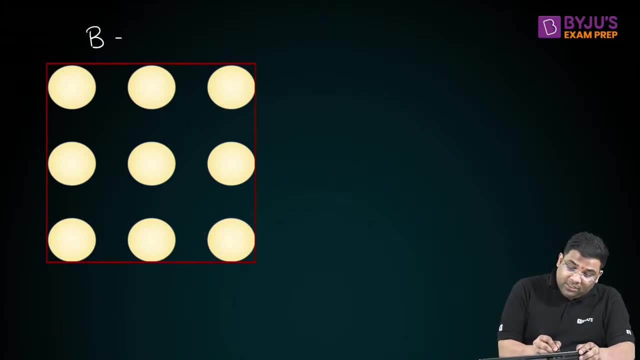 This is the thing. You see. it was so easy, right? If you know single pile in clay, you can easily find out for the group pile, right, Very easy. Now you see, when I am considering the block failure, then what will be this block size? This block size will be how much? I can say from your diagram, only 2S plus D. That is equal to 2.4 meter, because S was given 1 meter and diameter was given how much. 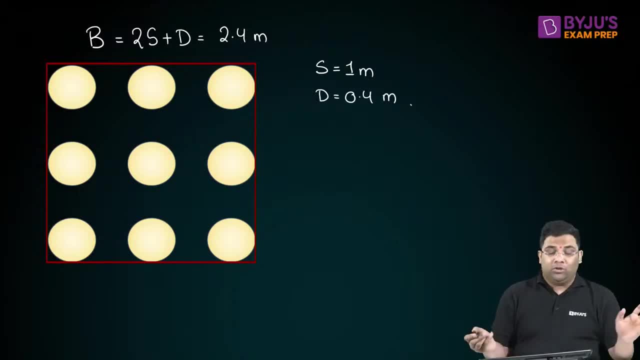 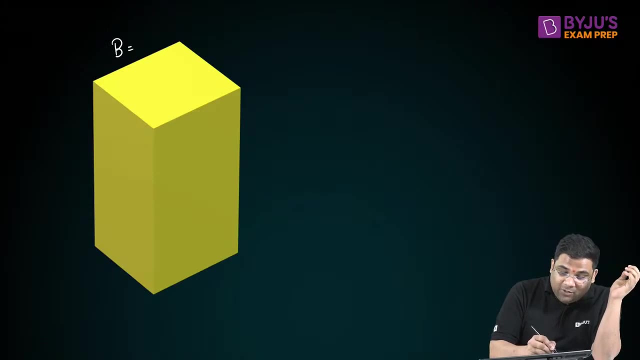 It was given. It was given to us as 4 meter, So the block size is 2.4. Now, if I have got that, the length is 20 meter. You see, you can easily now find out what You can easily now find out, that for this, the B you are getting is how much 2.4 meter. The length is 20 meter. Now you can find out the group capacity, considering block failure, as what Alpha will be 1 here. 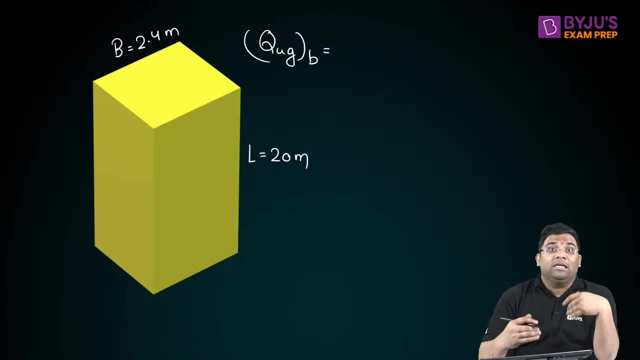 Alpha will be 1, right, Because now it is a block. Interaction will be what Clay and clay, So directly: C, that is your 40 into your 4, into B into L, right? The formula was what. The formula was: cohesion into the surface area. It is what: 4B into L, Then bearing capacity. 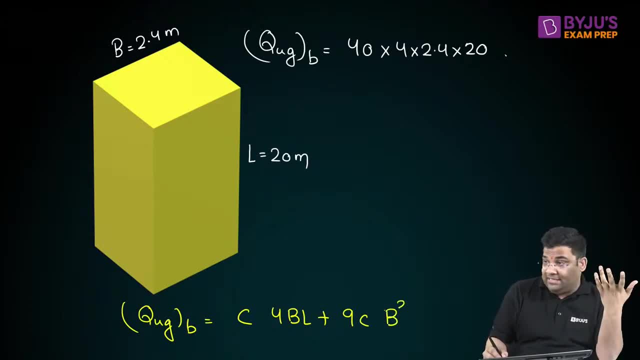 9C into surface area, is what Not surface area? Base area, is what B square? Salkar also found out the answer, So plus I can say: 9 into C, into B square, It is what 2.4 square? 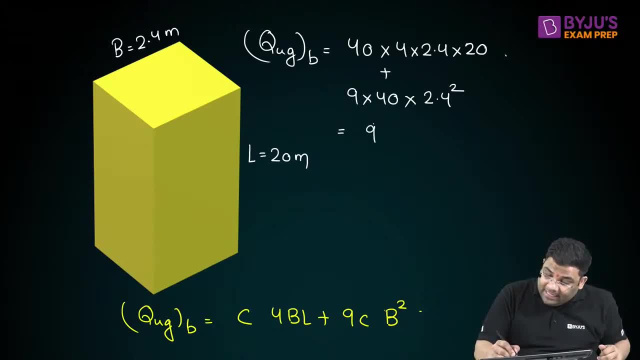 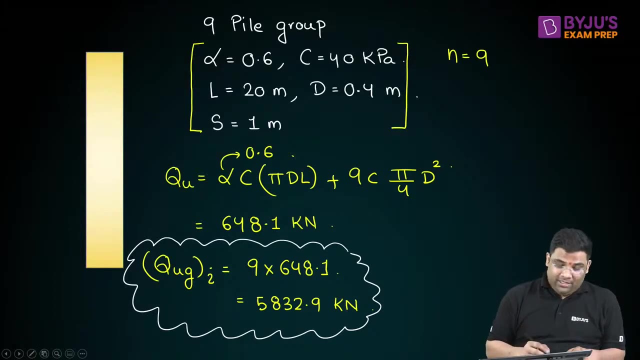 So how much I am getting. Others also found out 9753.6 kilonewton. So we got this answer right. This is so easy. If you know for individual pile, you can easily find out for group pile in clay. That is very easy, Not at all tough, okay. 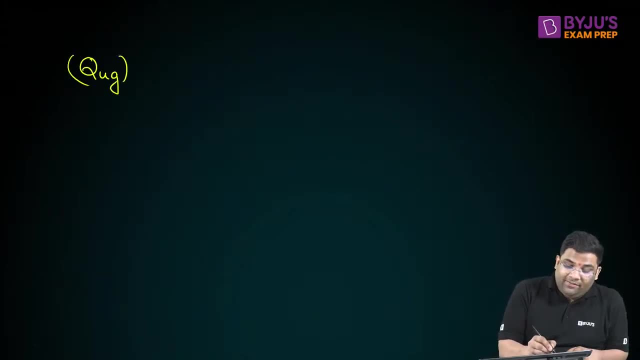 So I got that. the group capacity for individual failure is how much I got? that is 5832.9 almost. And for your group pile capacity, when I am considering block failure, I got how much: 9753.6 kilonewton. 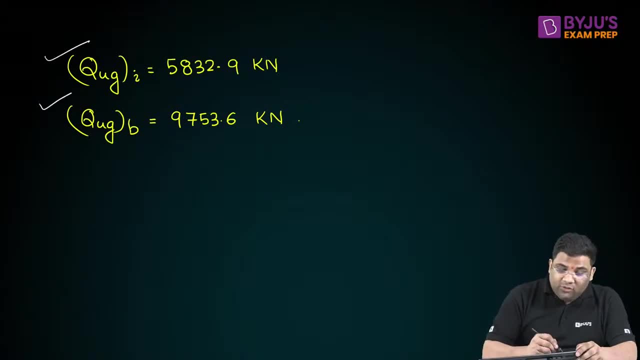 And these are the cases. okay, You will choose which one. Always you have to choose the minimum one. okay, The minimum one you should choose, and that will be that. what That group capacity of the pile group, Okay, say, ultimate capacity of the pile group, group capacity also I can say, So it will be how much: 5832.9 kilonewton. 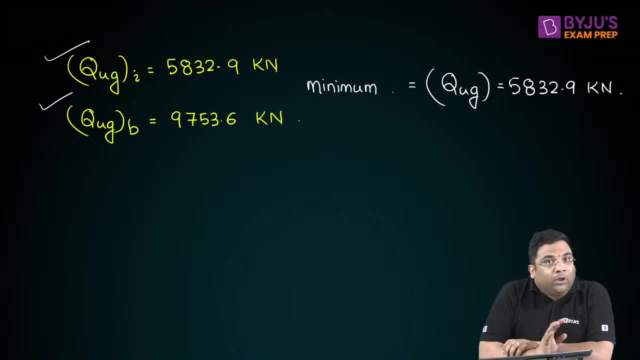 Very good, Very good students, So thank you very much for all the students So attentively attending the class. yes, and obviously you are getting benefited. So this is one of the most important topics for your pile foundation. okay, Most important topics for the pile foundation. We saw three things right. 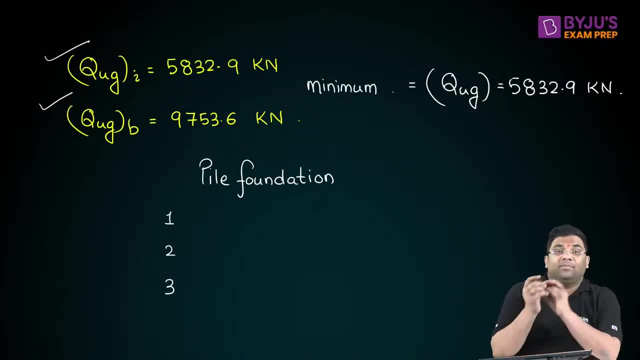 First one was what Single pile in single layer- Okay, Okay, Okay, Okay, Okay Okay. Single pile in multilayer. Then, finally, we saw what Group of piles- Okay, Group of piles. So thank you very much. 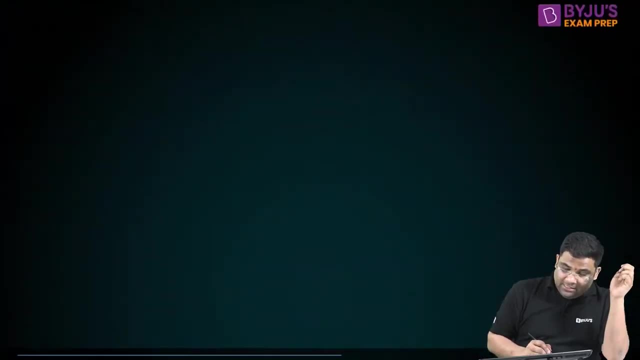 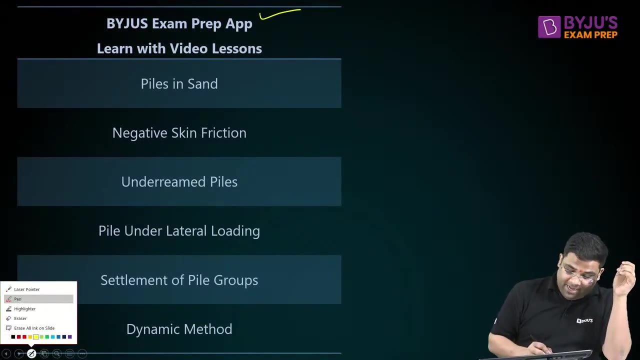 So let us see that there are some other topics which I have taught in your Byju's exam prep. If you go to your Byju's exam prep and then you go to your learn with video lessons in geotech and under the chapter pile foundation, there are some other important topics. 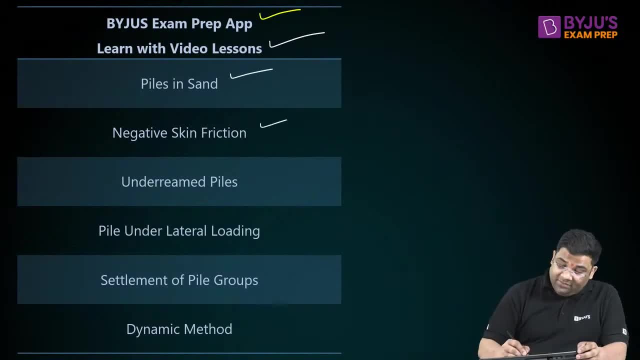 And then again you have students in enormellow class. the pile structure picture: yes, That is what Pile in sound negative screen friction, underrimmed piles pile under lateral loading. then settlement of pile groups and dynamic method. 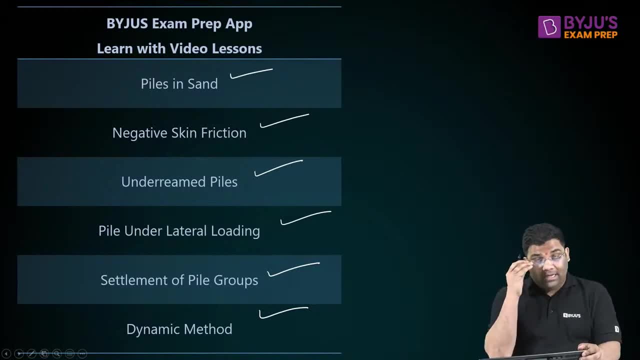 So all these things I have taught in the Byju's exam prep app, learn with video lessons. Go and see yourself. if you have any doubts, you can message to my number. Okay, now tomorrow's lecture. Okay, Okay, Okay.